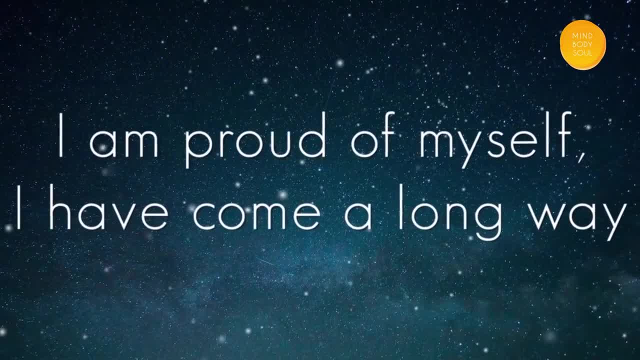 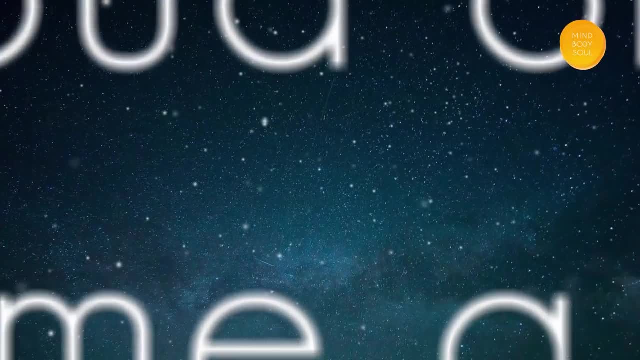 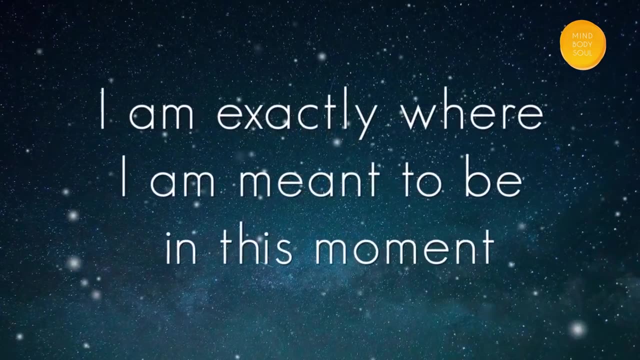 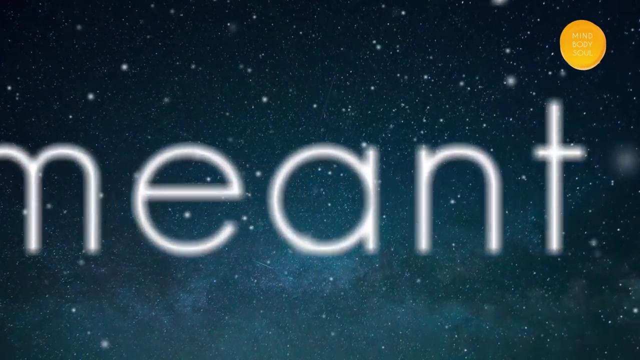 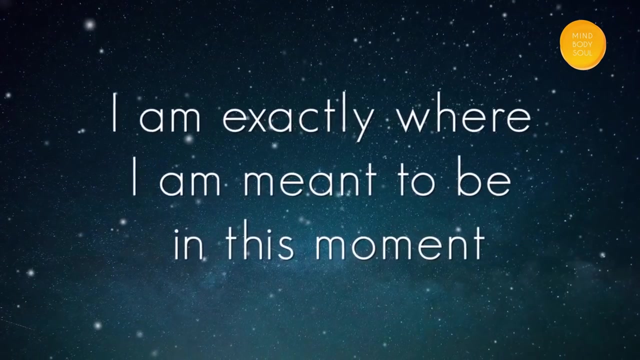 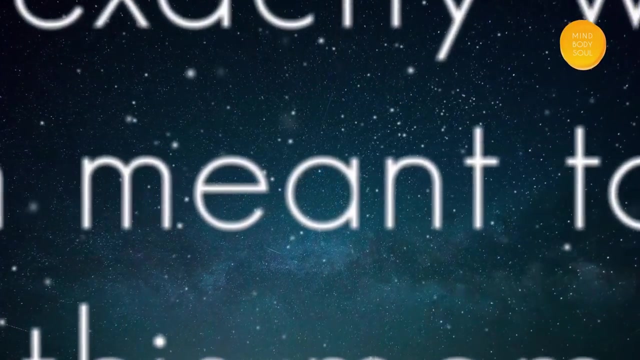 I am proud of myself. I have come a long way. I am proud of myself. I have come a long way, a long way. I am exactly where I am meant to be in this moment. I am exactly where I am meant to be in this moment. 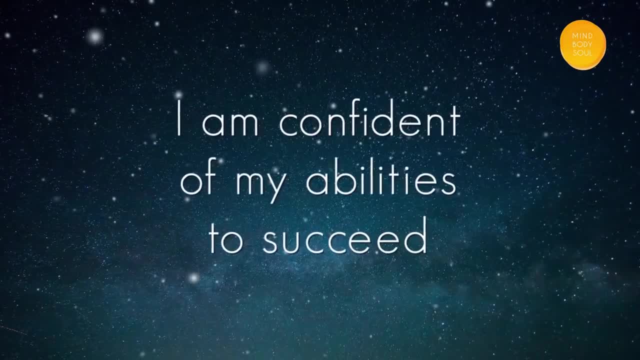 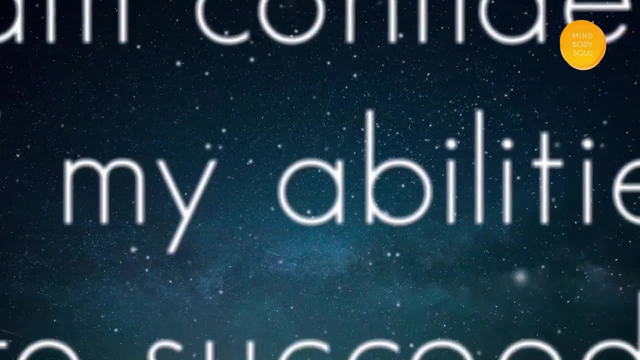 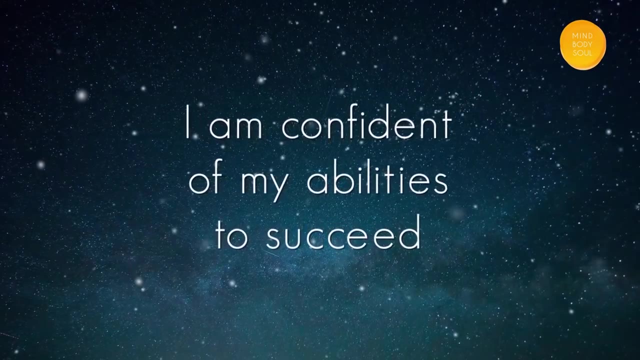 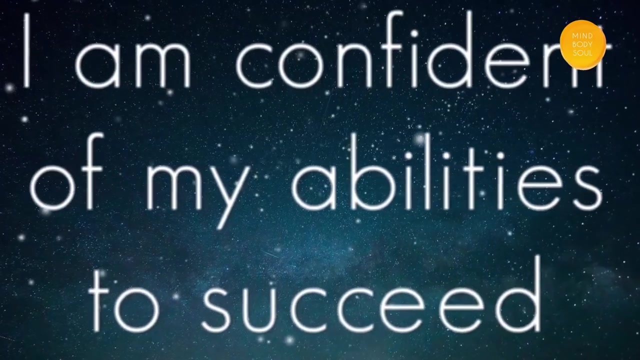 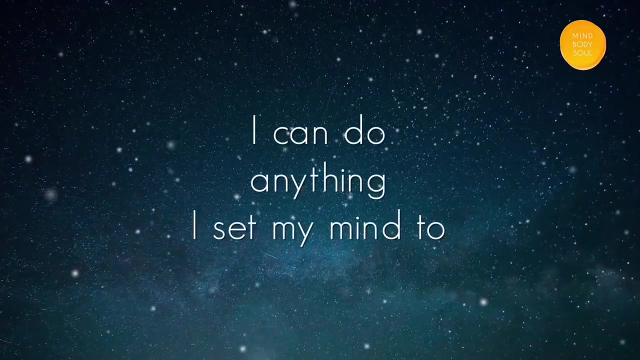 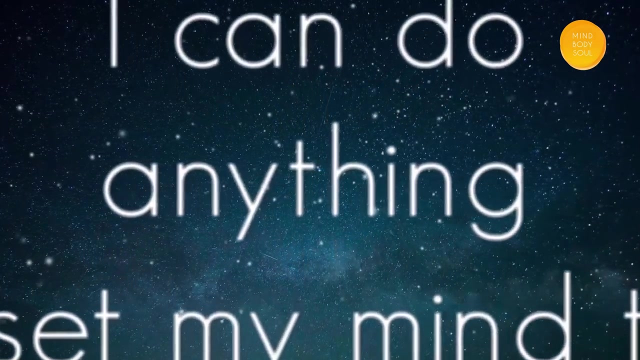 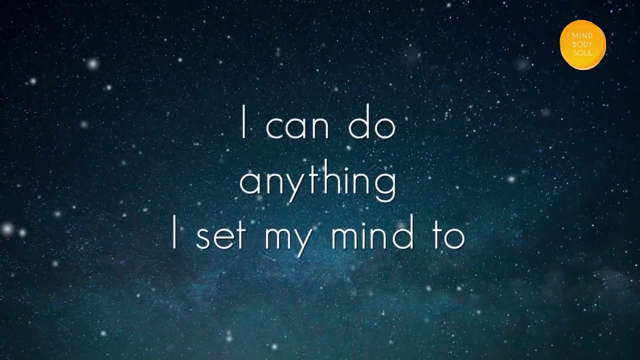 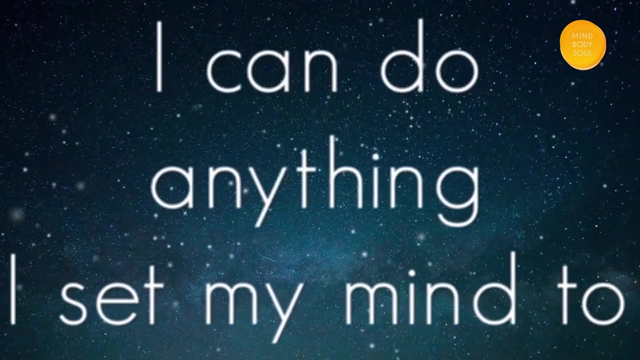 I am confident of my abilities to succeed. I am confident of my abilities to succeed. I can do anything I set my mind to. I can do anything I set my mind to. I can do anything I set my mind to, Anything I set my mind to. 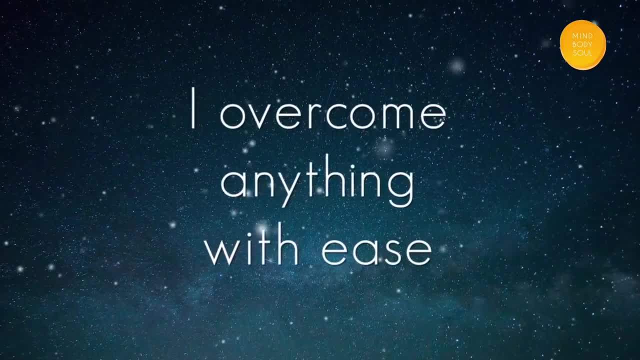 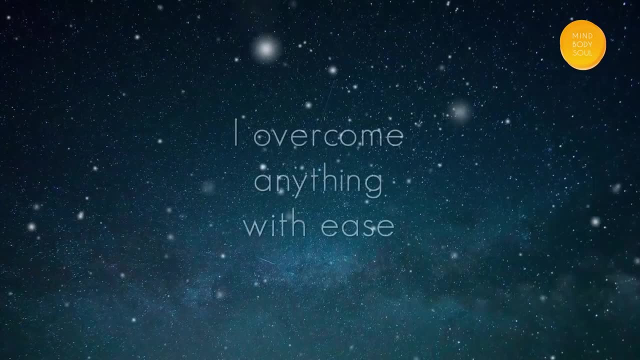 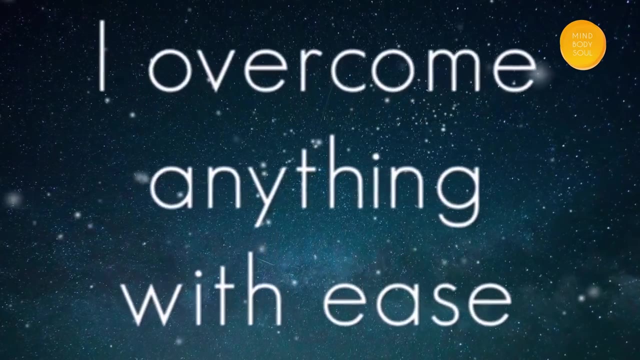 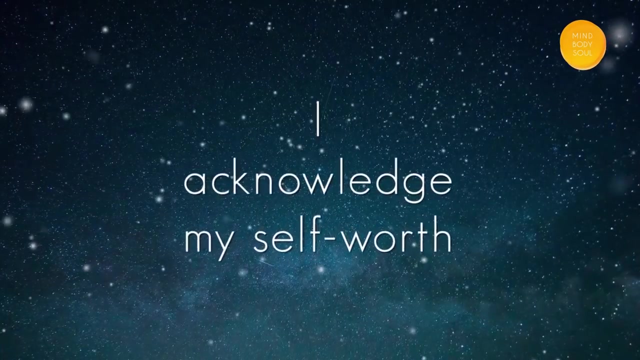 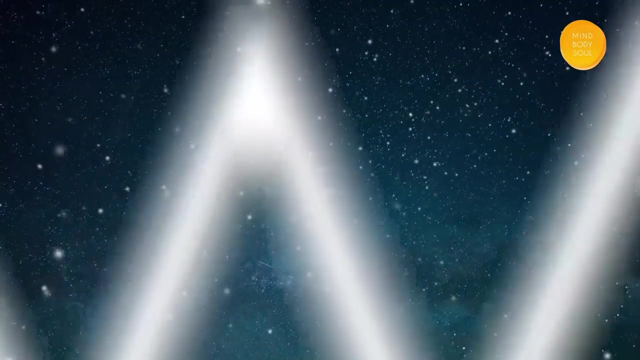 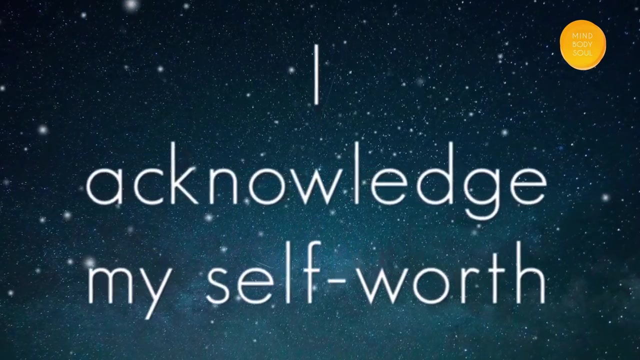 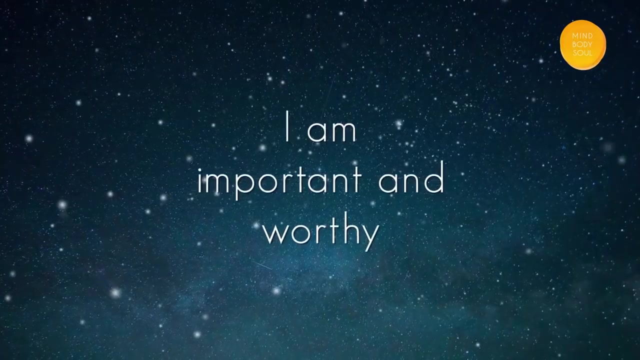 I overcome anything with ease. I overcome anything with ease. I acknowledge my self-worth. I acknowledge my self-worth. I acknowledge my self-worth. I am important and worthy. I am important and worthy. I am important and worthy. 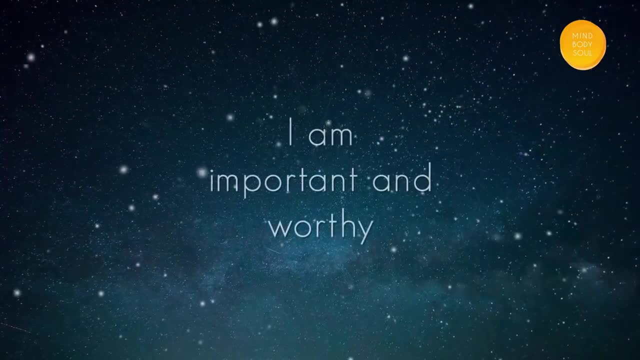 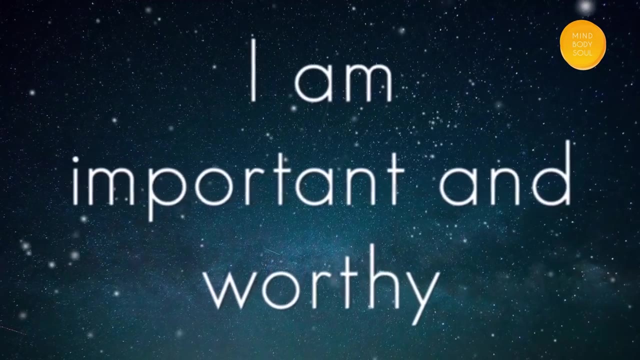 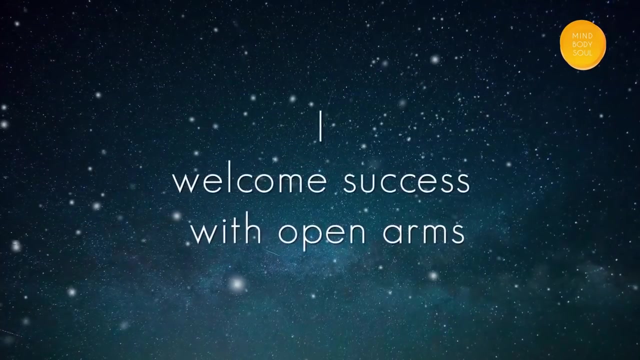 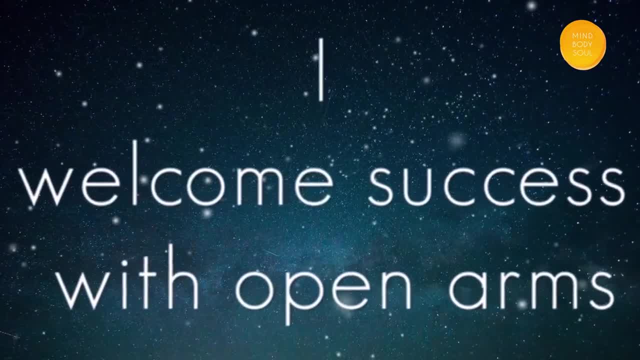 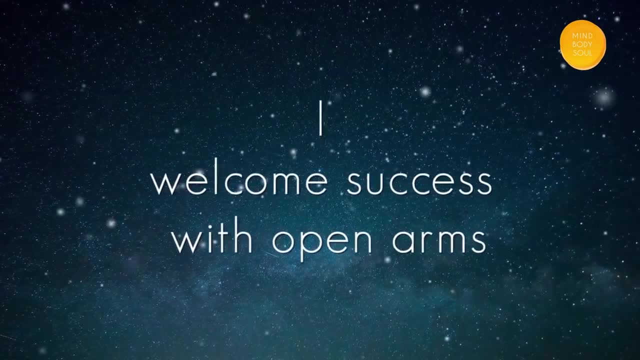 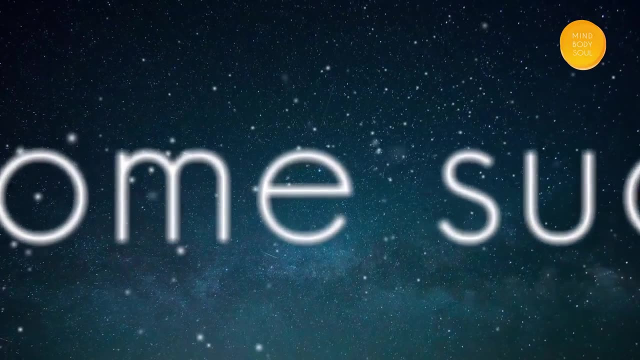 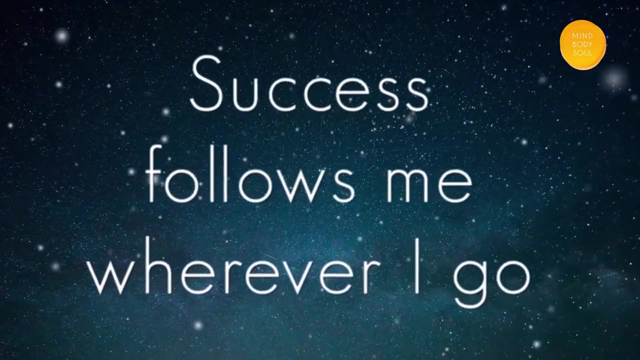 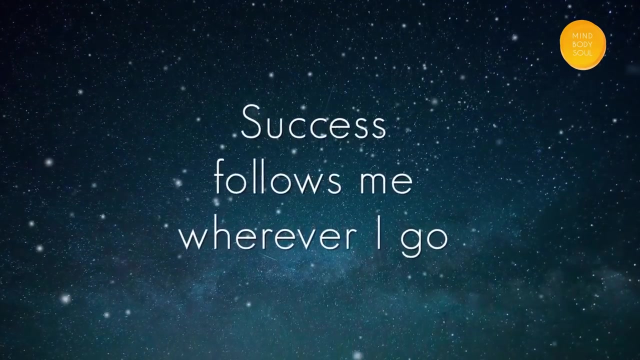 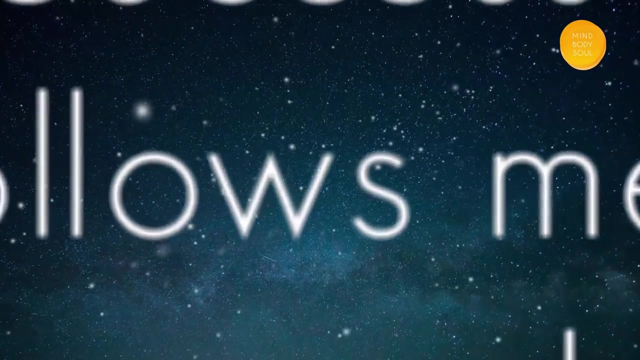 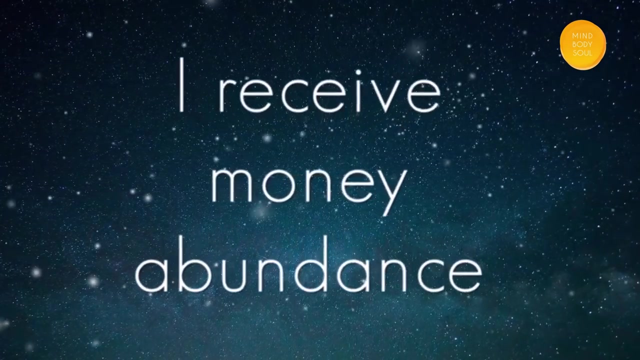 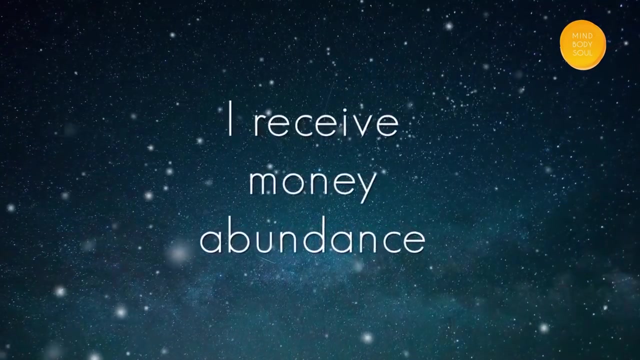 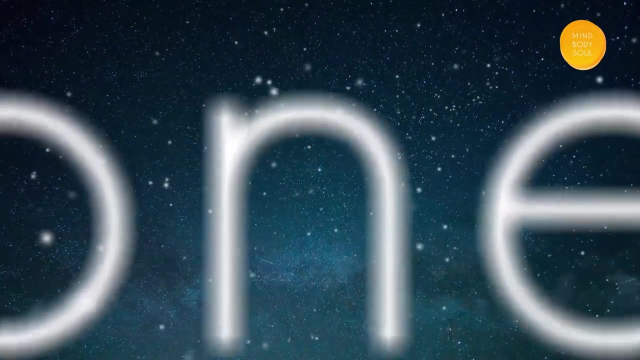 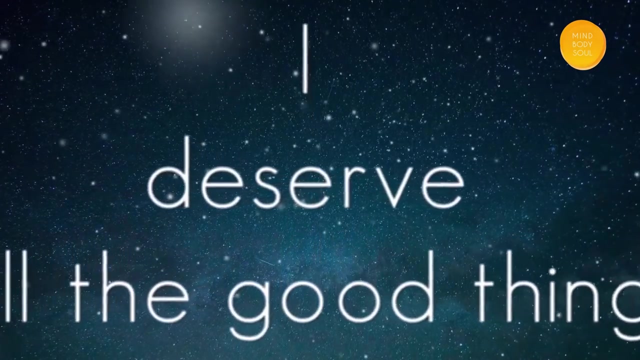 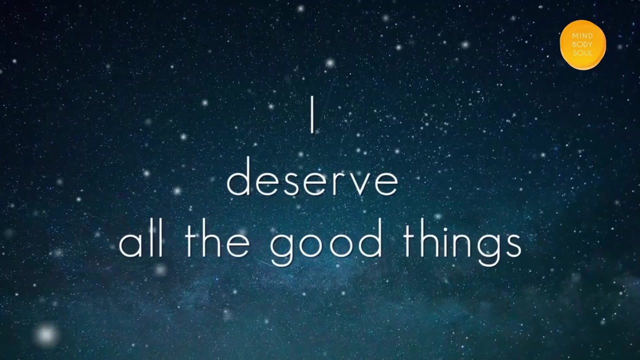 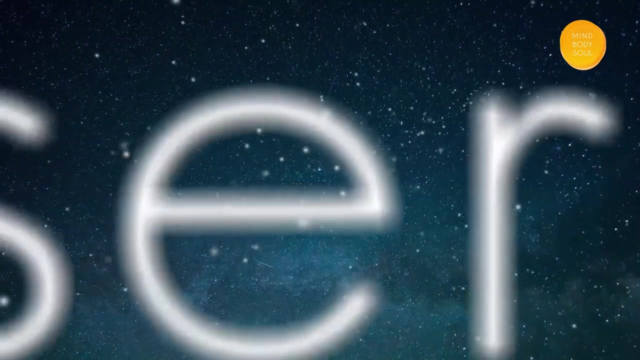 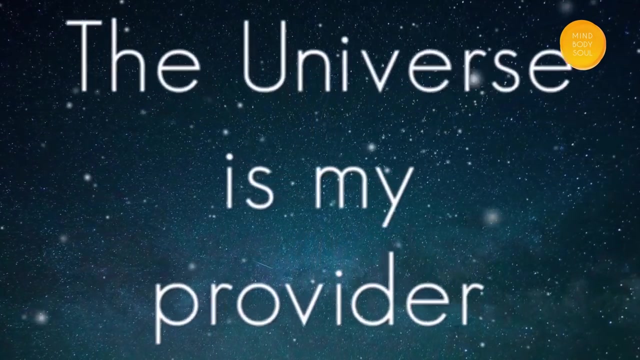 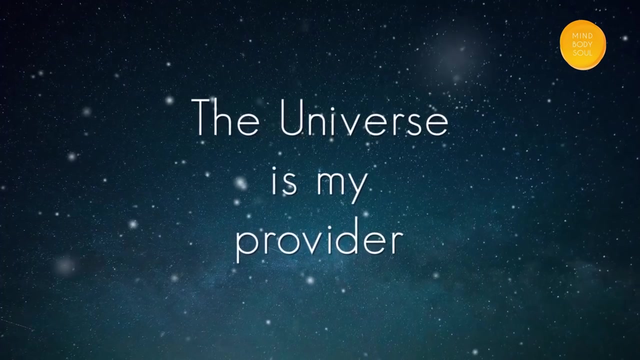 with open arms. I welcome success with open arms. success follows me wherever I go. success follows me wherever I go. I receive money abundance. I receive money abundance. I deserve all the good things. I deserve all the good things. the universe is my provider. the universe is my provider. 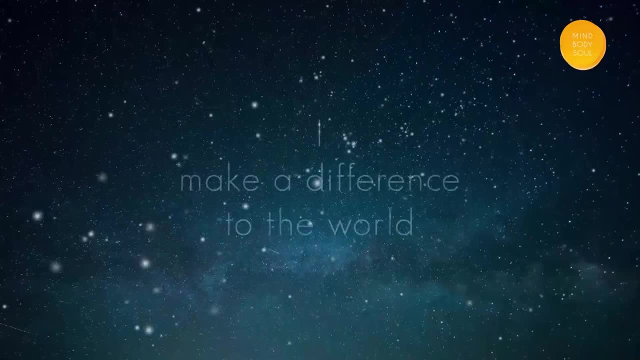 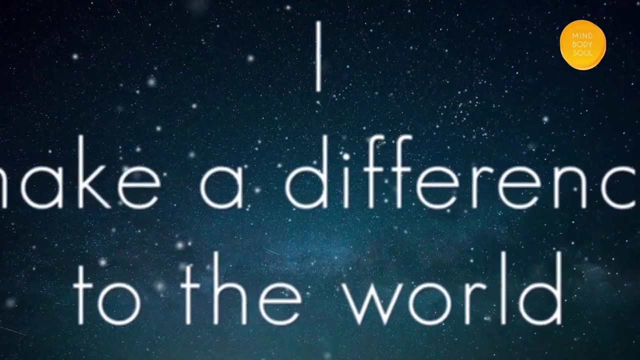 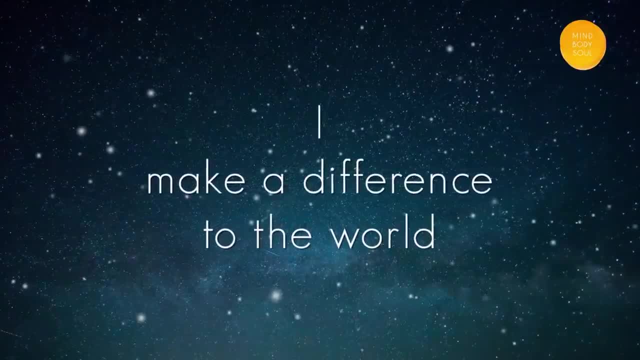 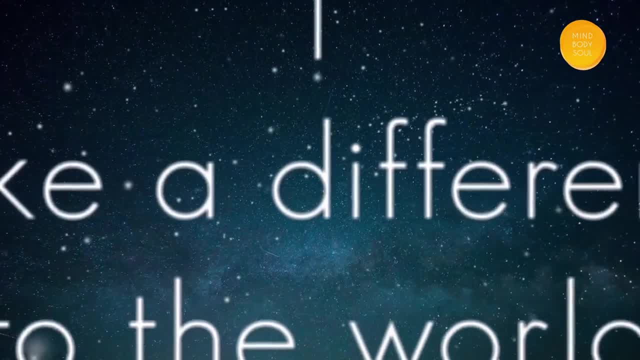 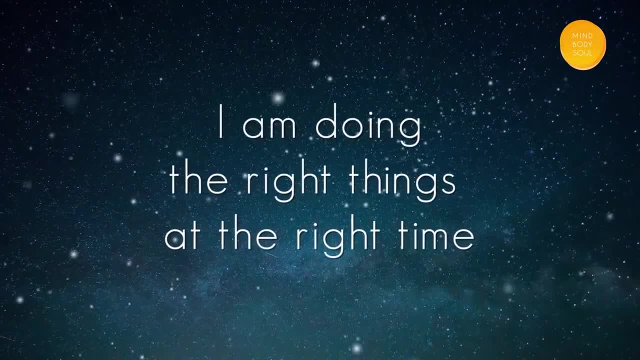 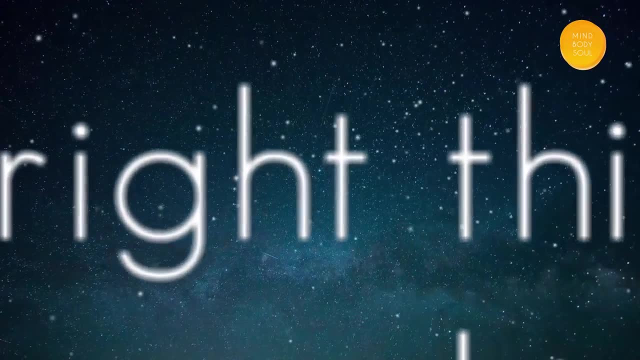 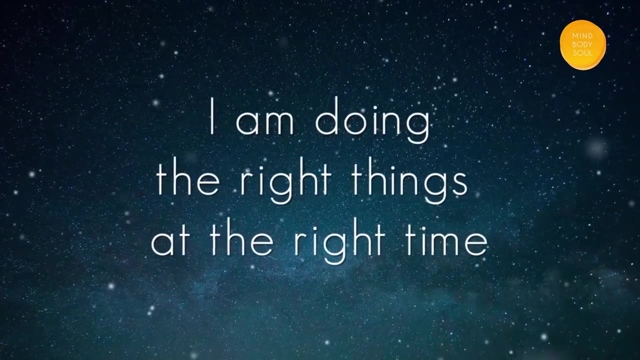 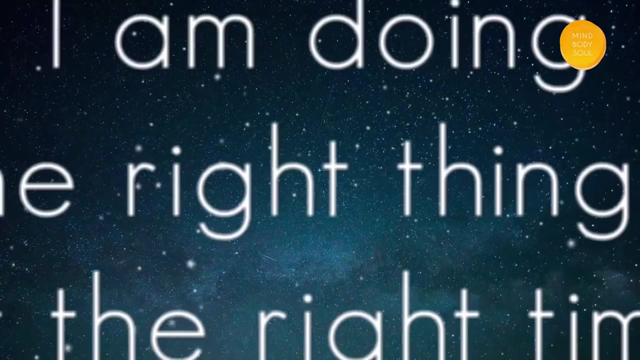 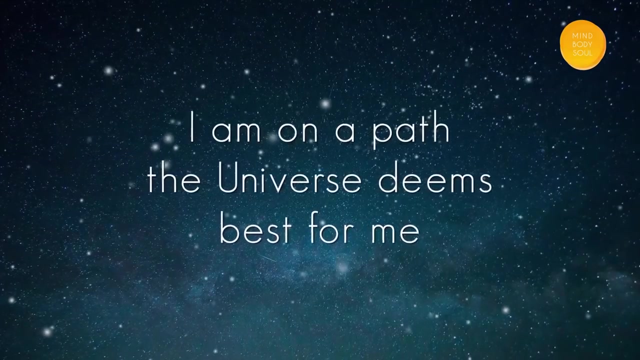 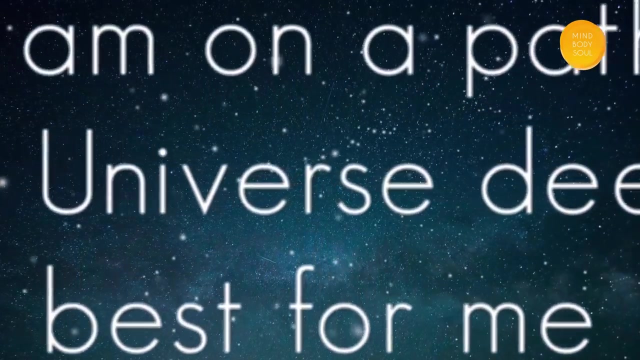 I am doing the right things at the right time. I am doing the right things at the right time. doing the right things at the right time. I am doing the right things at the right time. I am on a path the Universe deems best for me. 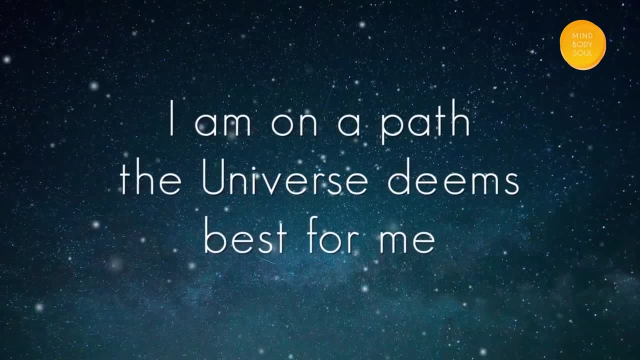 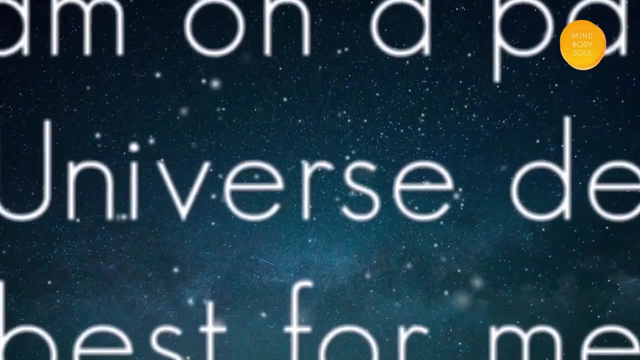 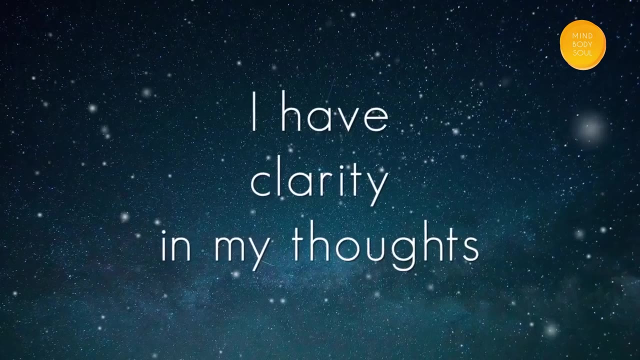 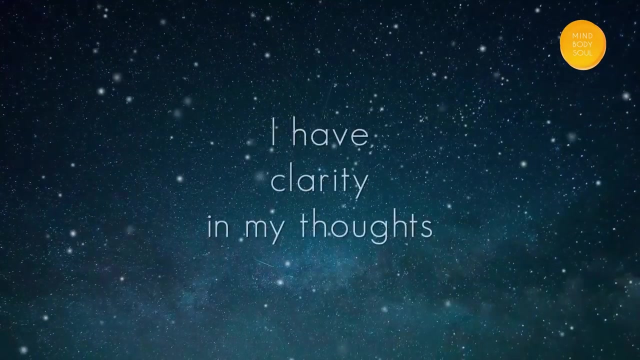 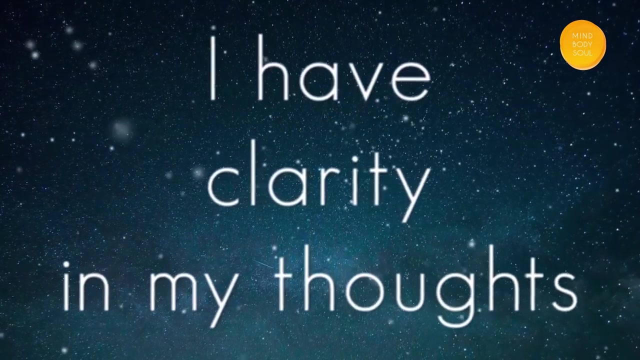 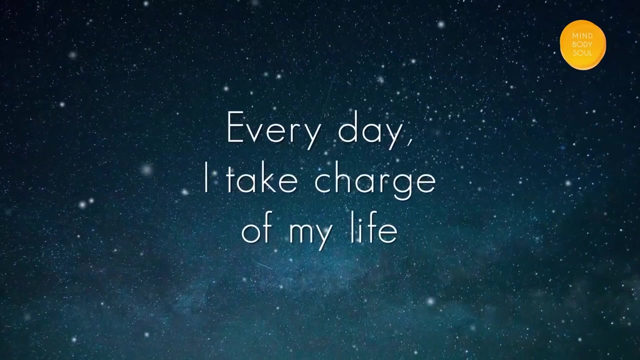 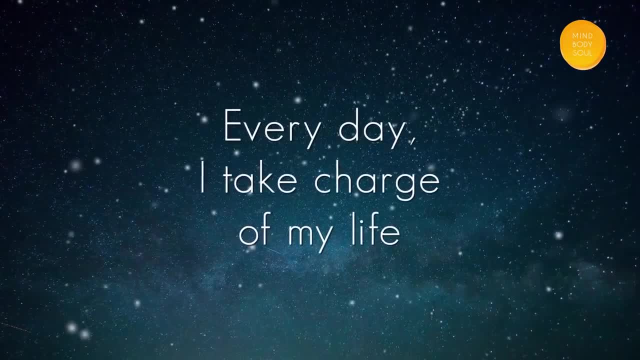 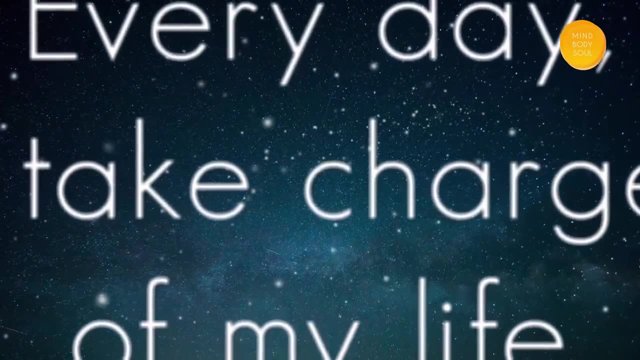 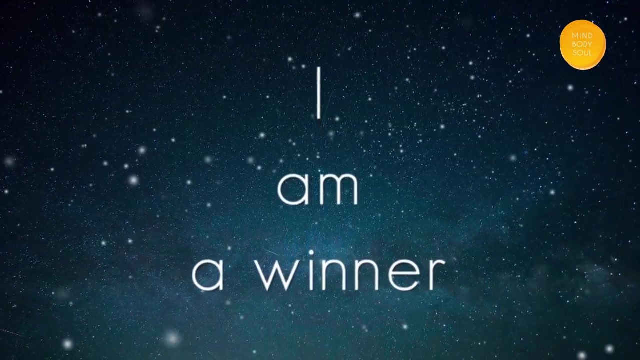 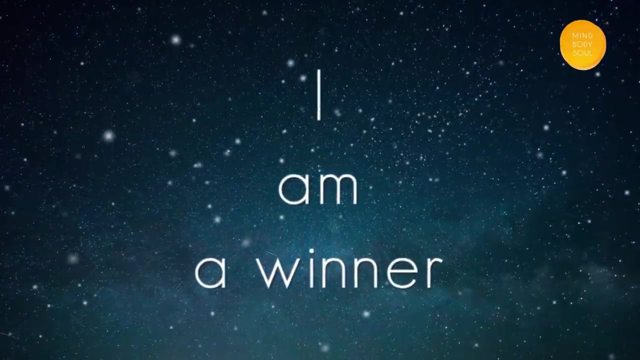 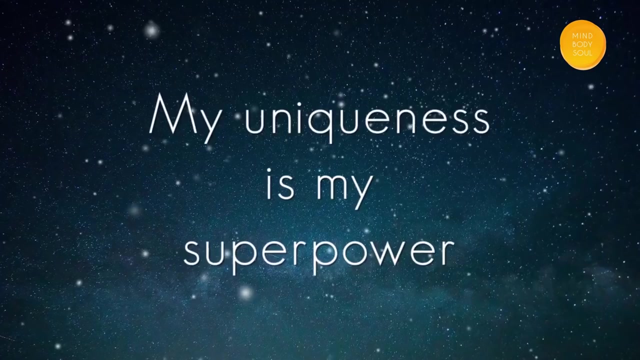 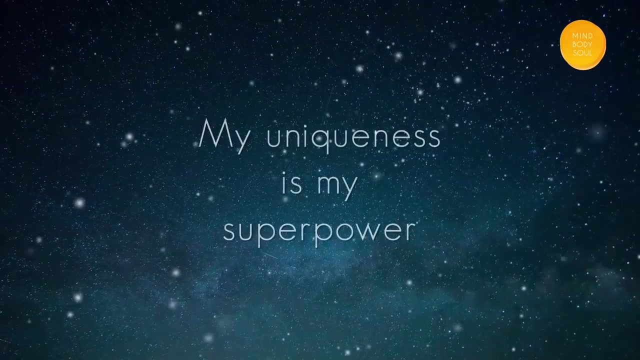 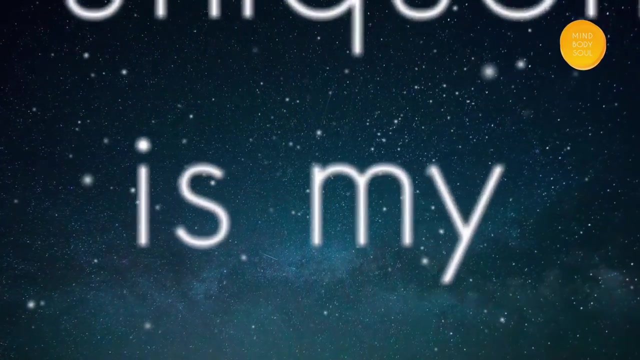 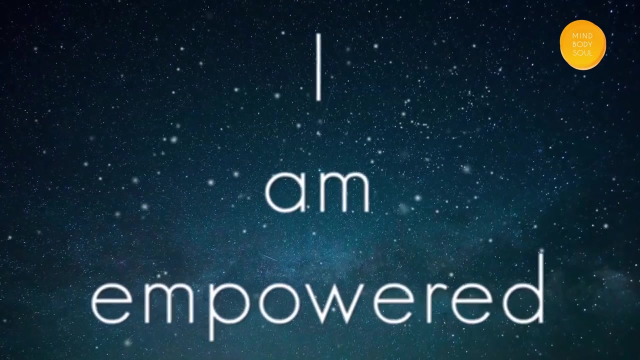 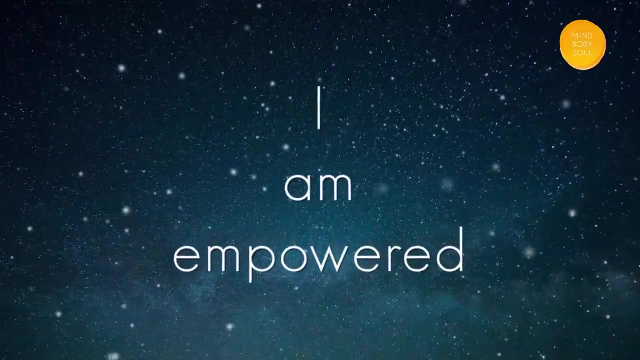 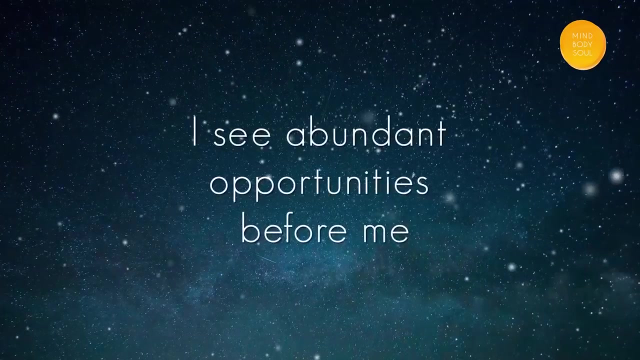 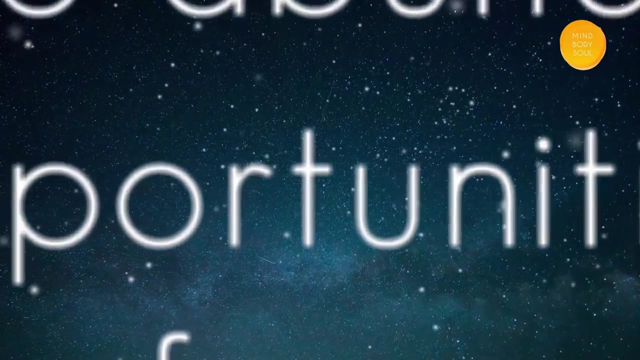 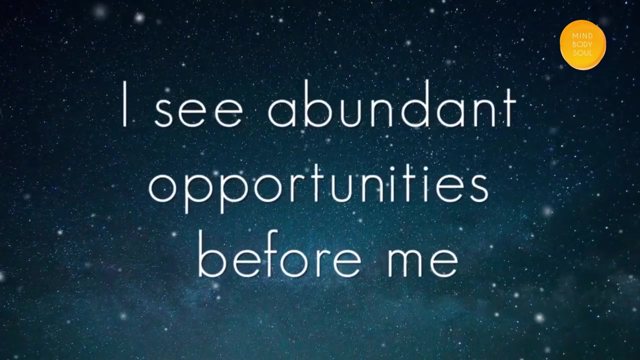 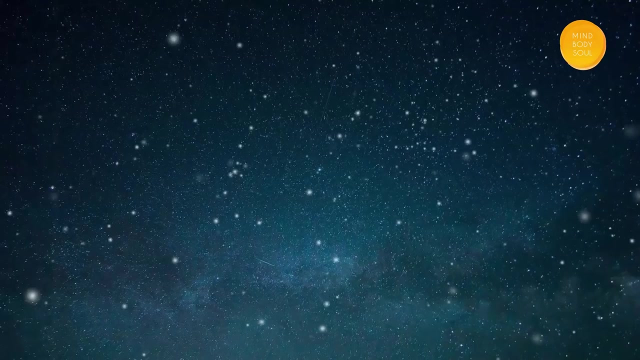 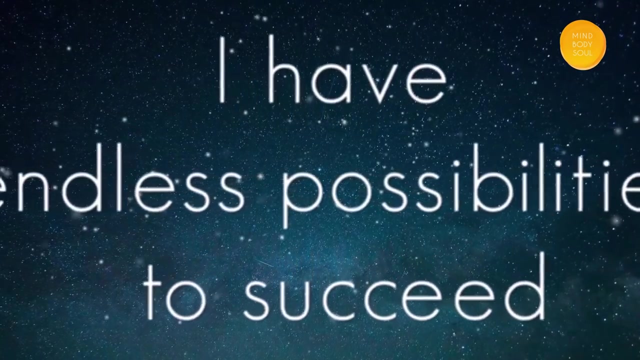 every day, I take charge of my life. I am a winner. I am a winner. my uniqueness is my superpower. my uniqueness is my superpower. I am empowered. I am empowered. I see abundant opportunities before me. I see abundant opportunities before me. I have endless possibilities to succeed. 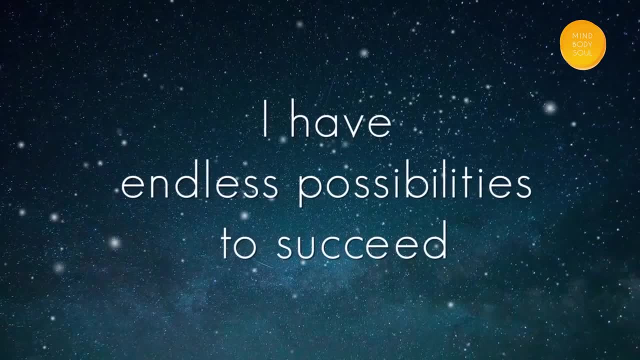 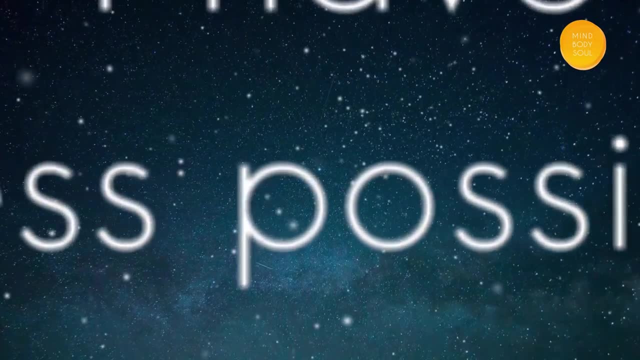 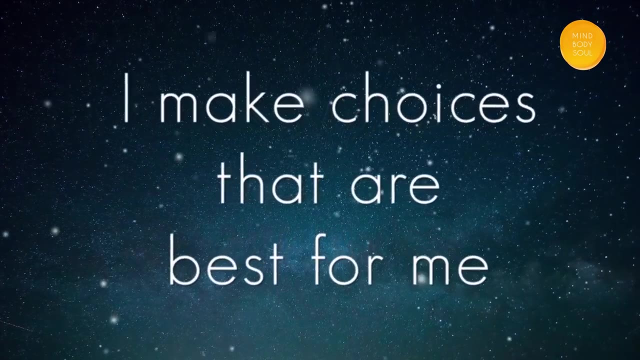 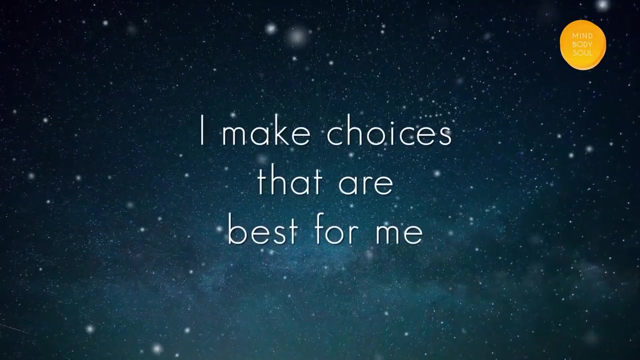 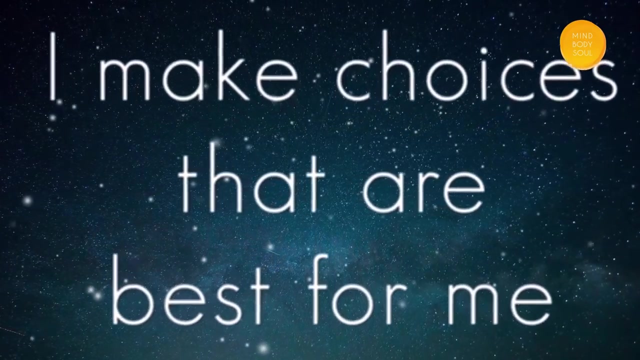 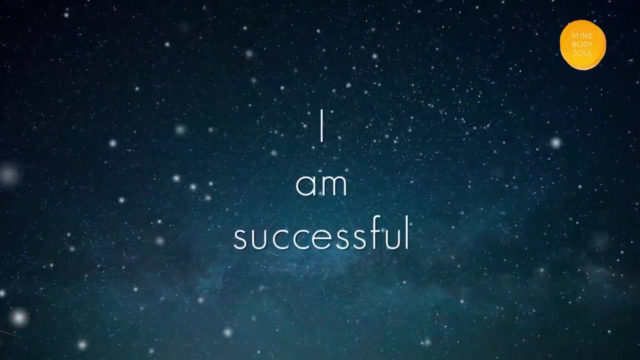 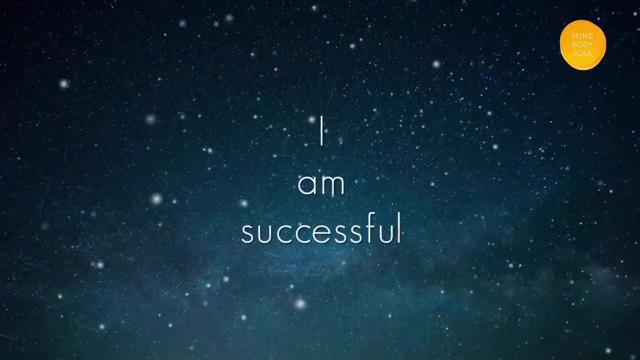 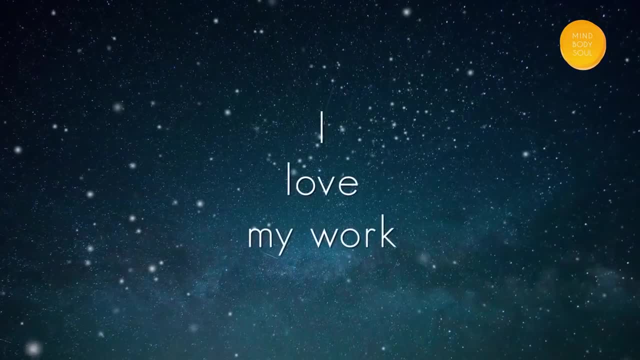 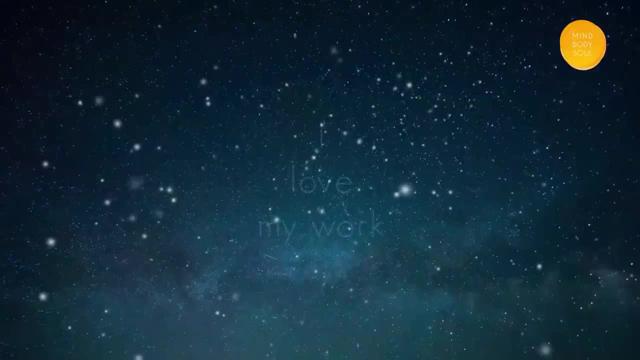 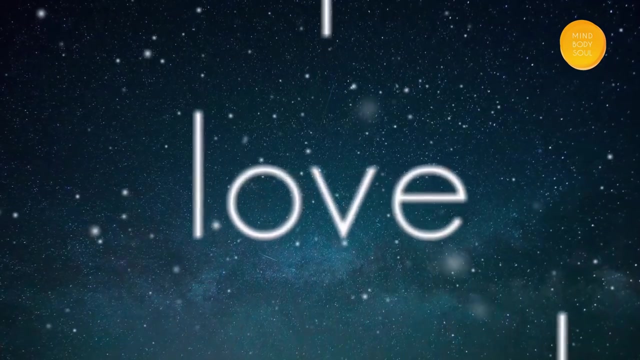 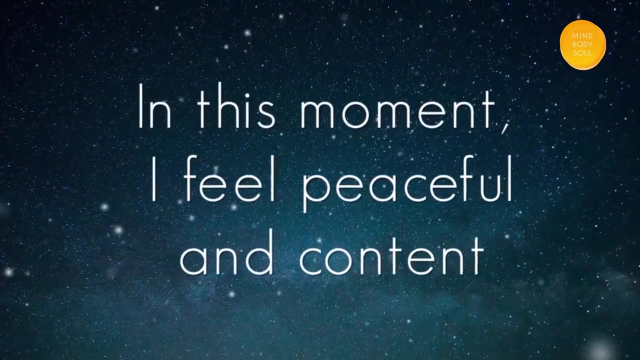 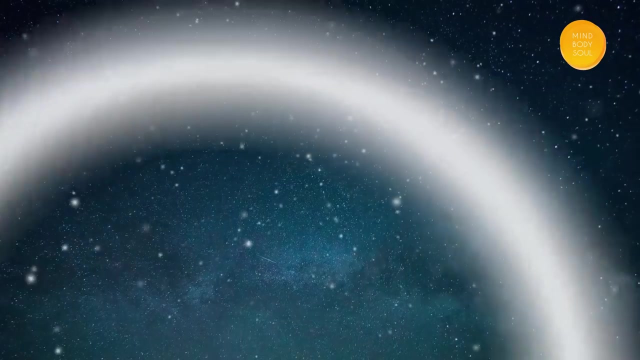 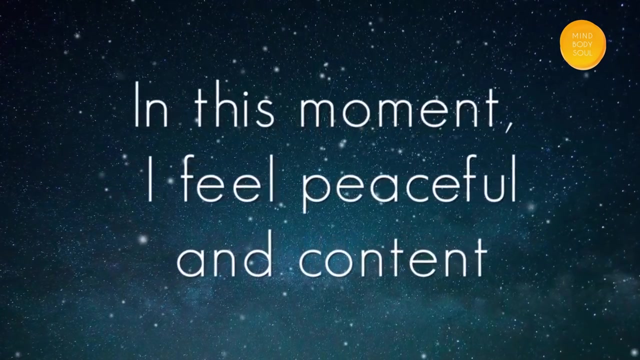 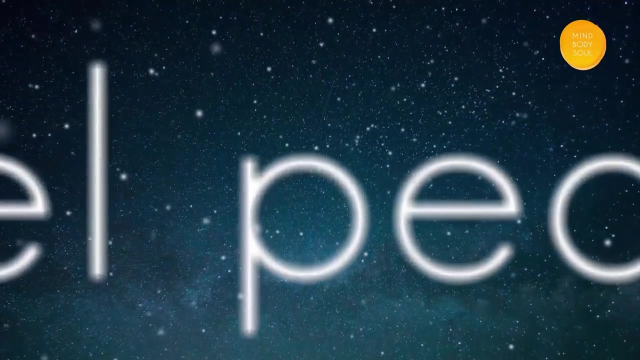 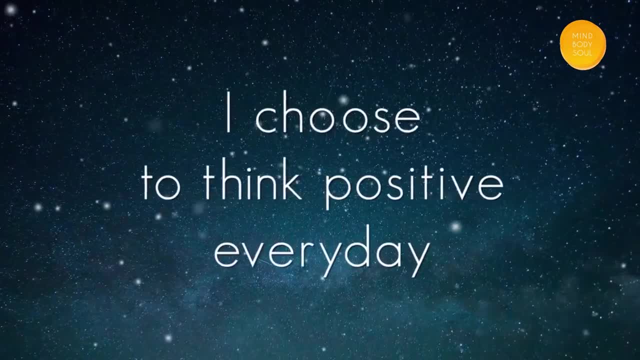 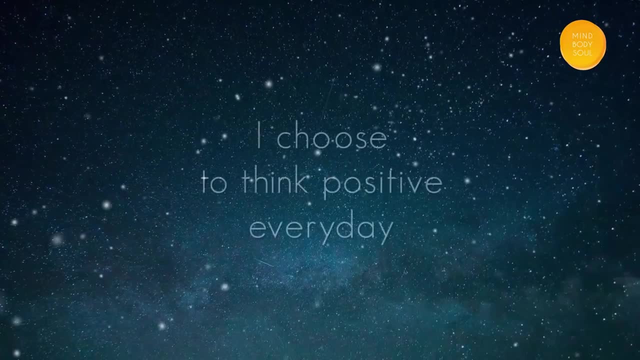 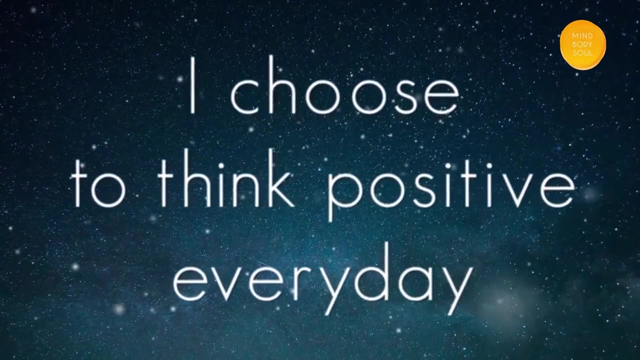 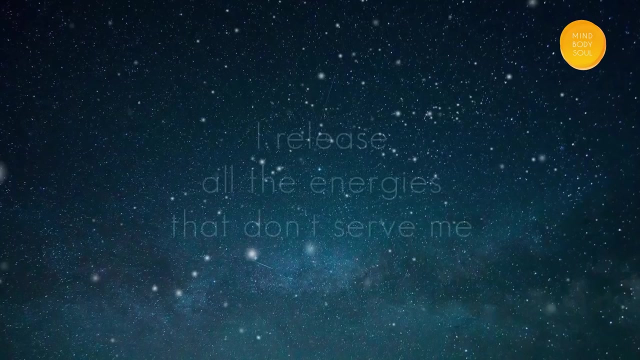 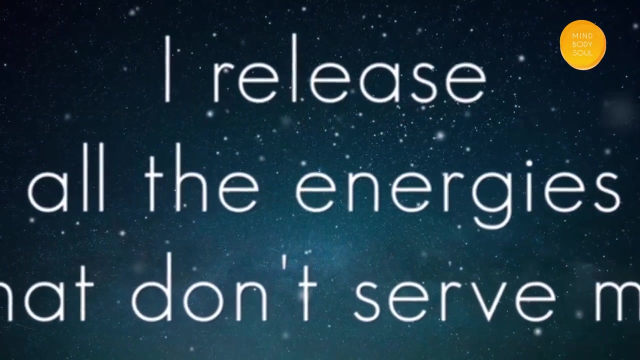 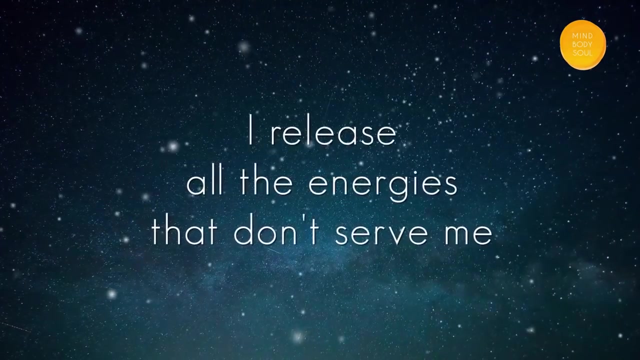 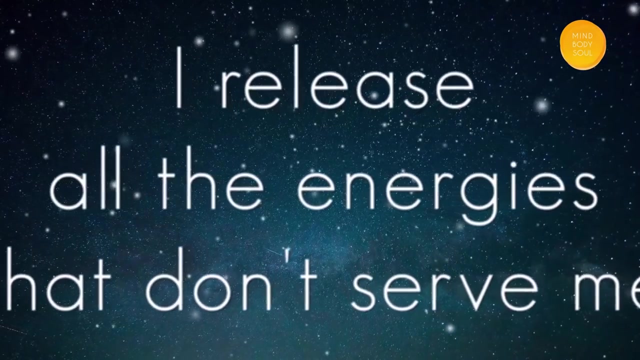 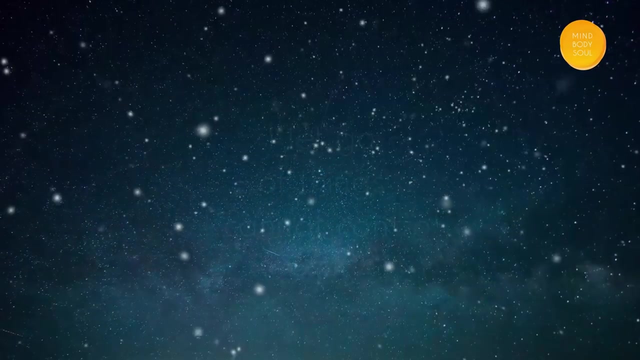 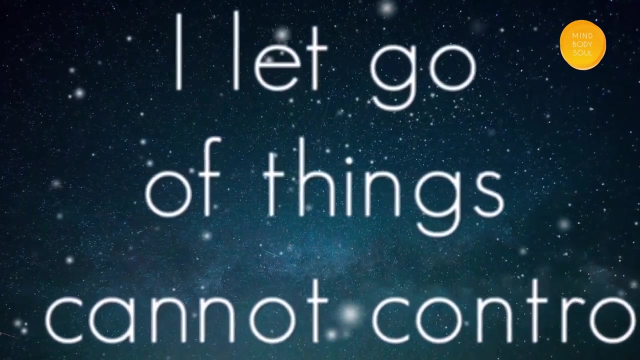 I choose to think positive every day. I release all the energies that don't serve me. I release all the energies that don't serve me. I let go of things I cannot control. I let go of things I cannot control. I let go of things I cannot control. 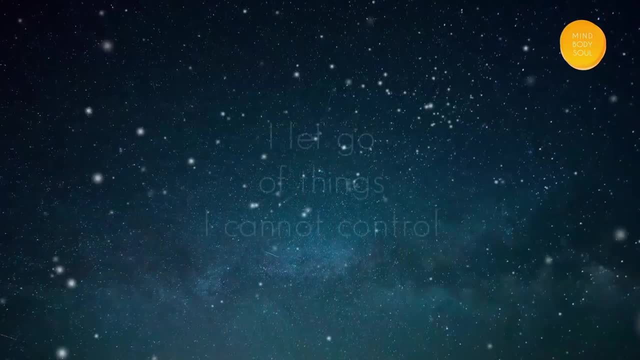 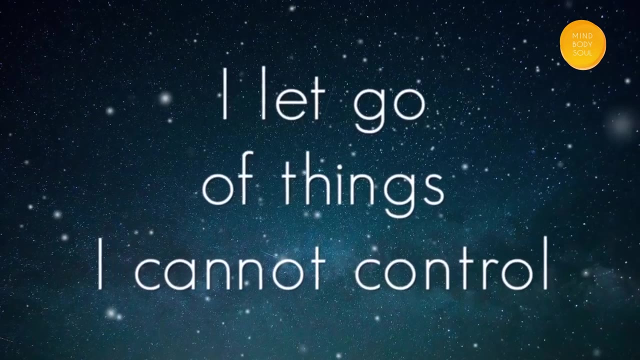 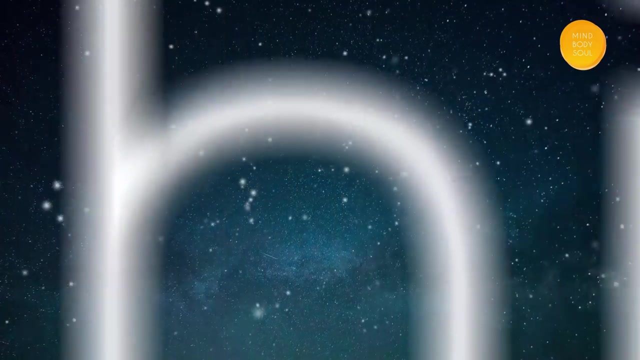 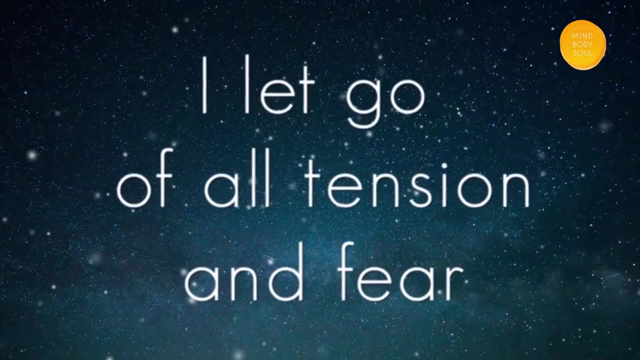 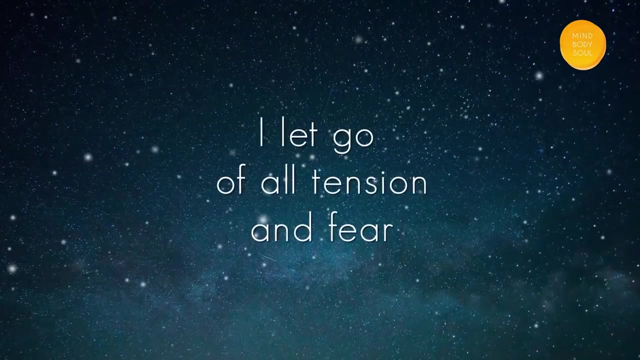 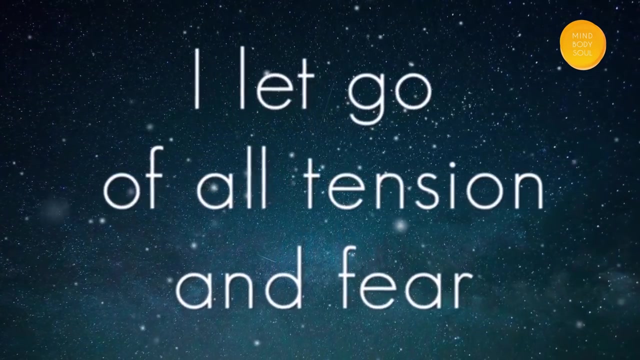 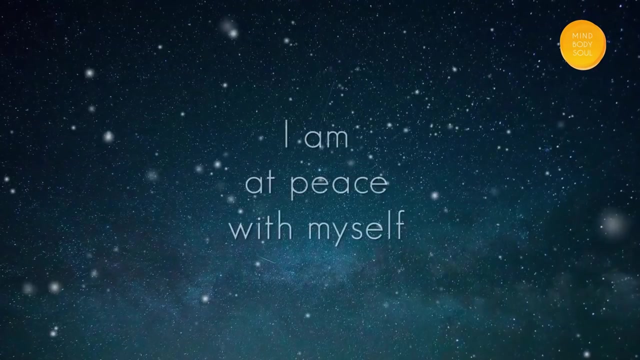 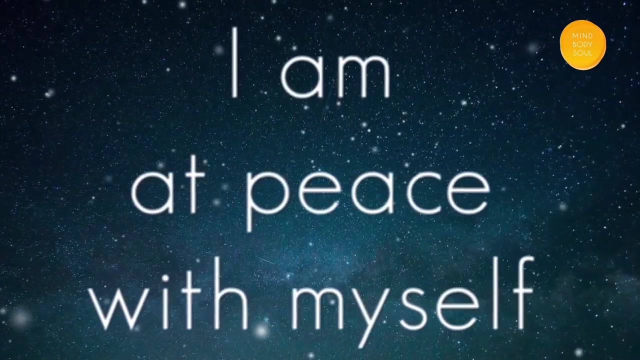 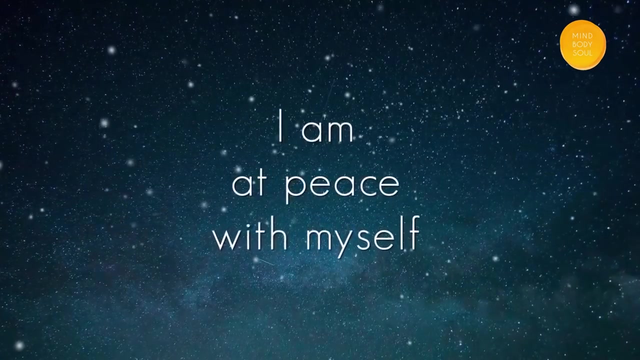 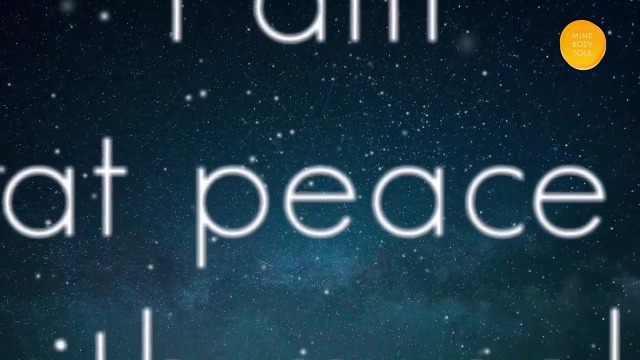 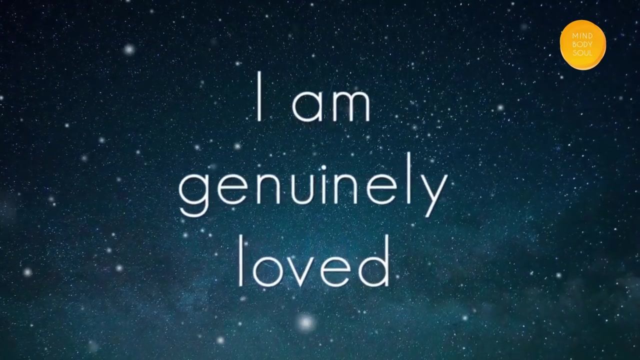 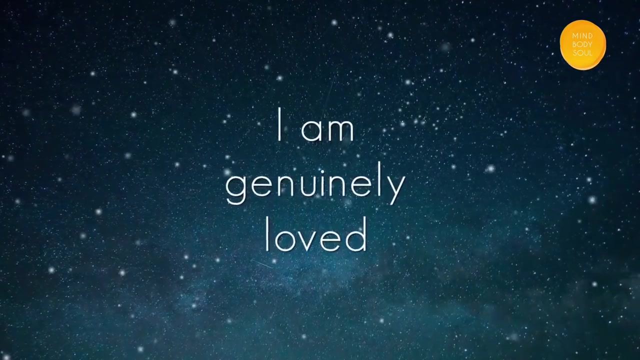 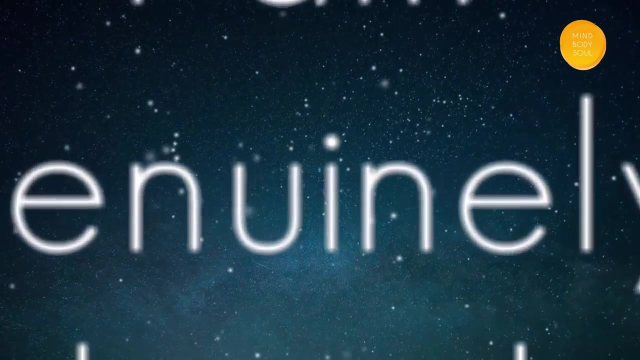 I let go of all tension and fear. I let go of all tension and fear. I let go of all tension and fear. I am at peace with myself. I am at peace with myself. I am genuinely loved. I am loved. I am genuinely loved. I am loved for who I am. 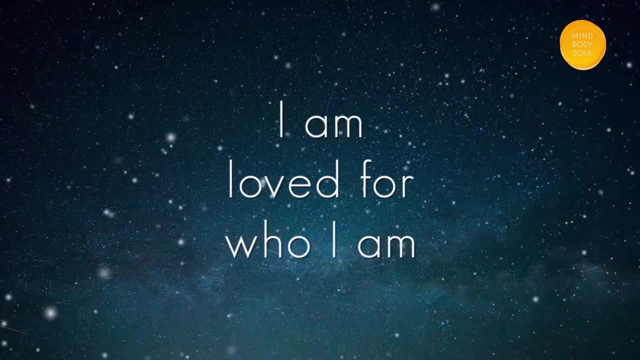 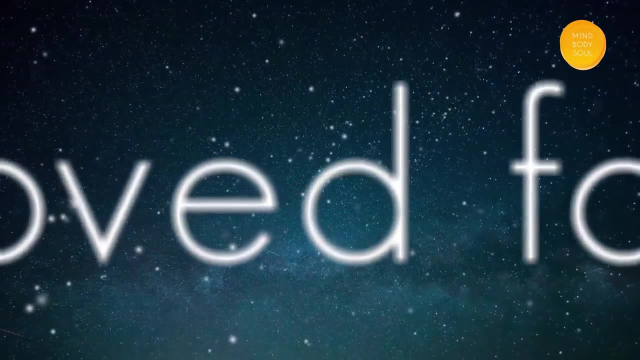 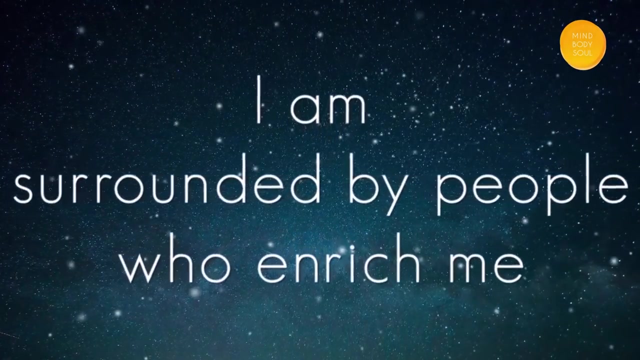 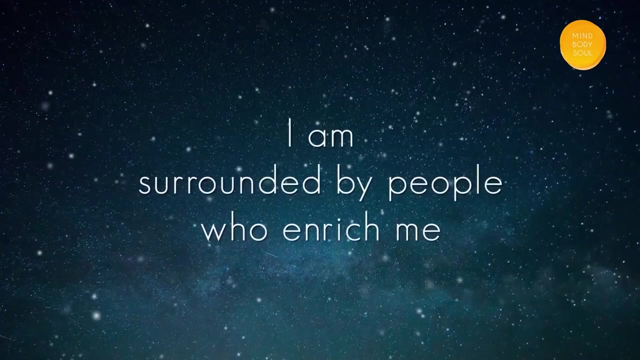 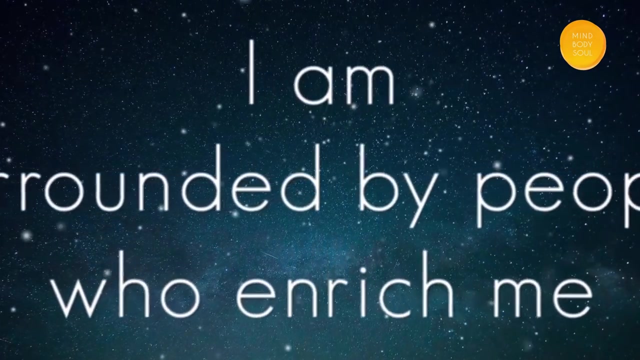 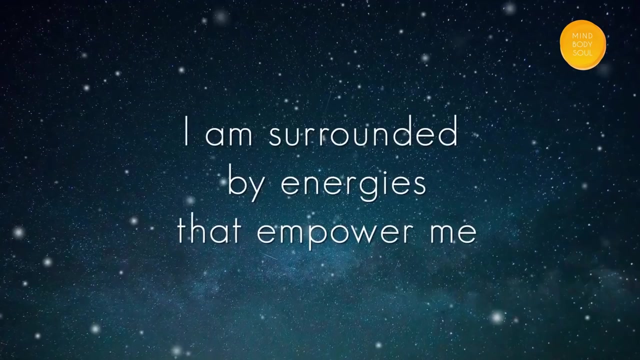 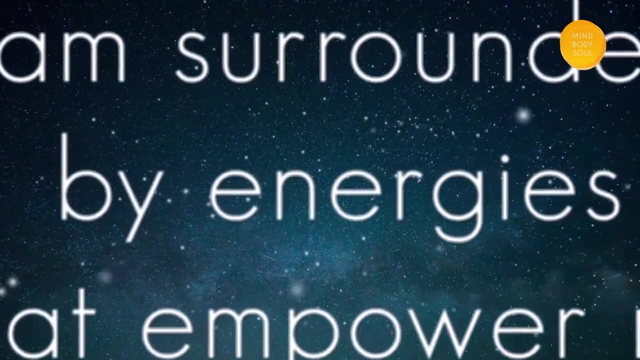 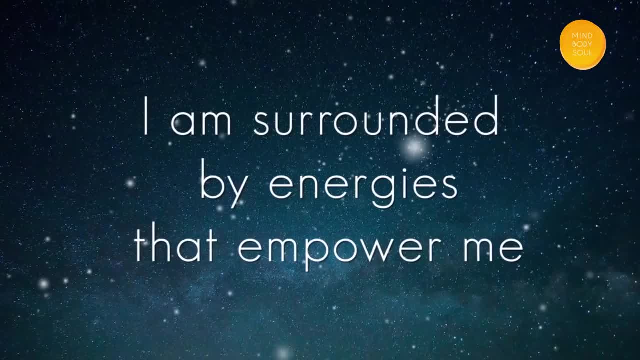 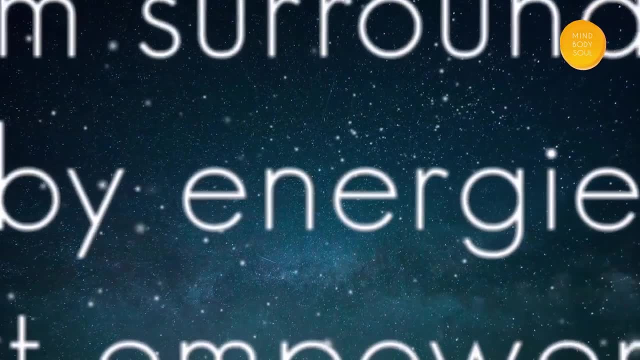 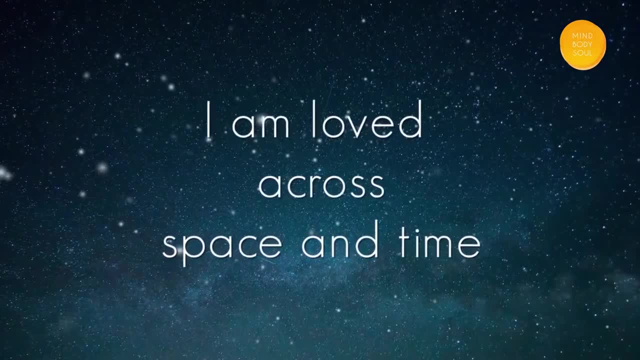 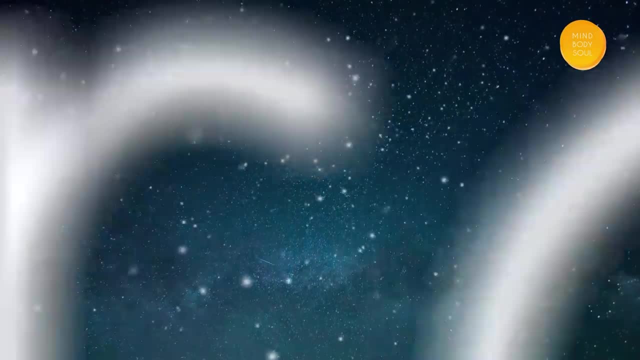 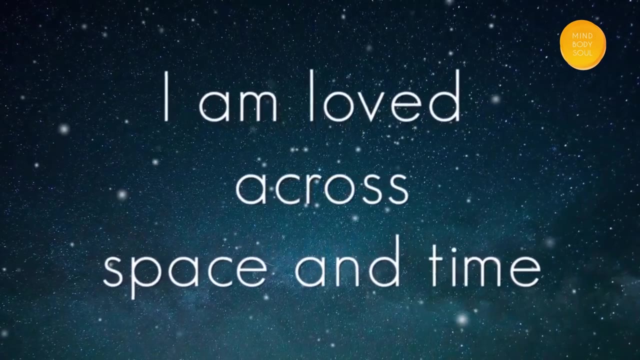 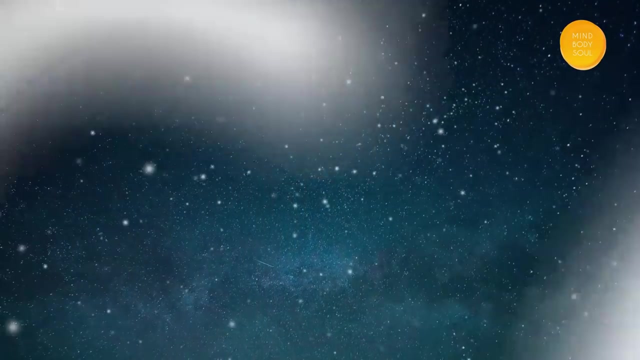 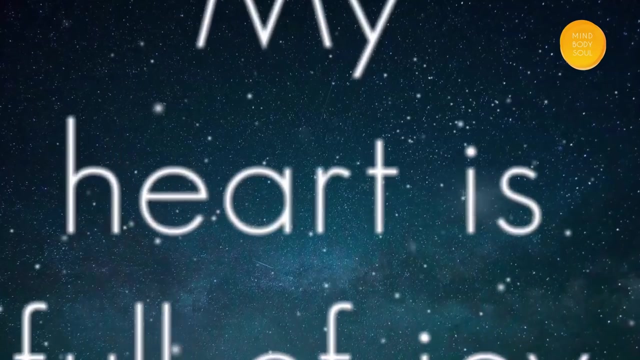 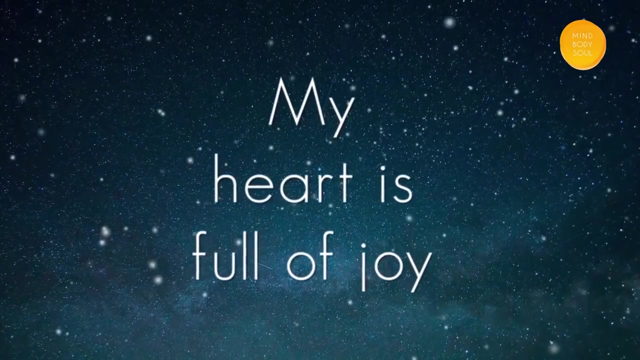 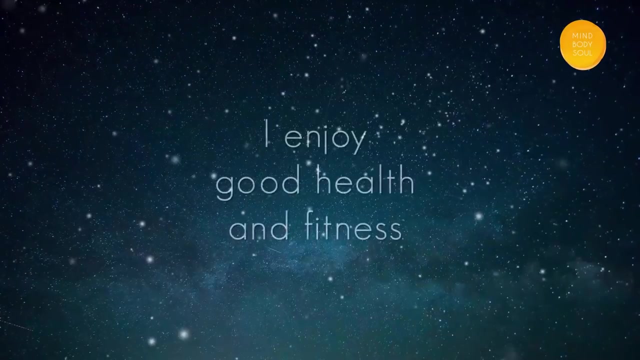 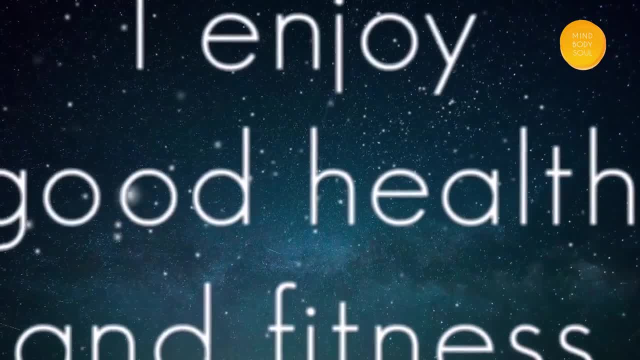 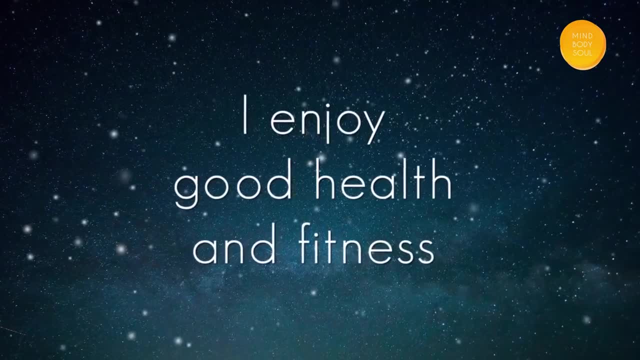 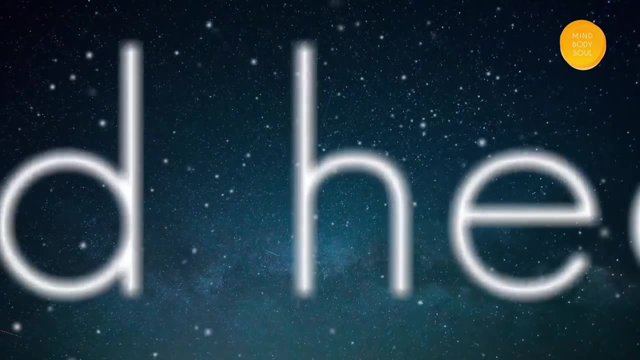 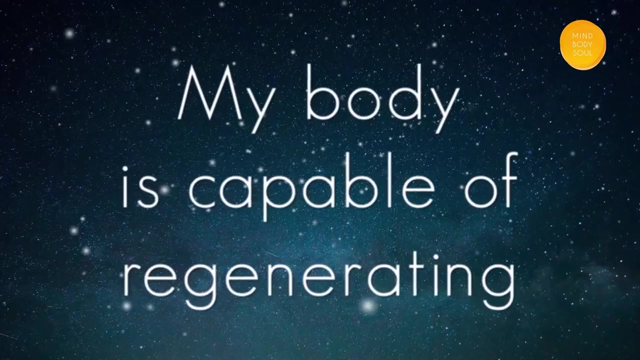 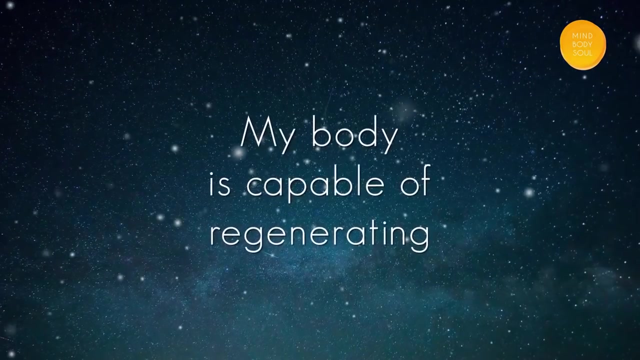 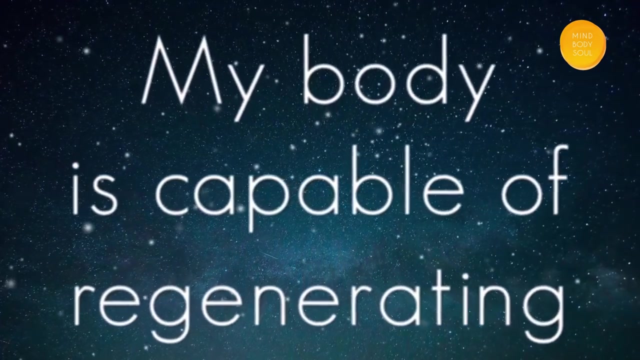 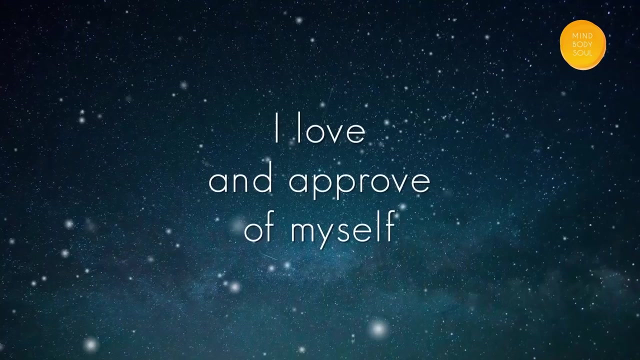 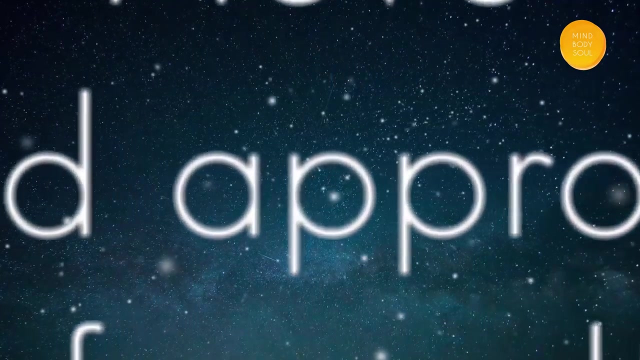 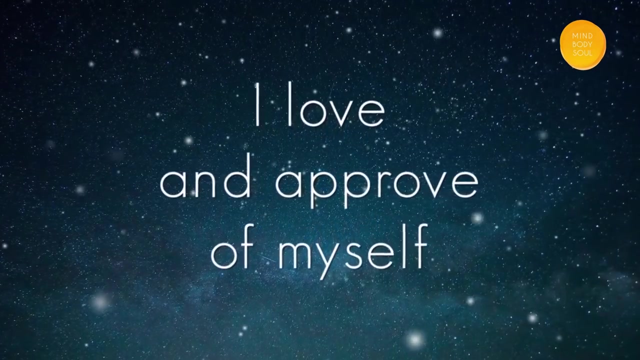 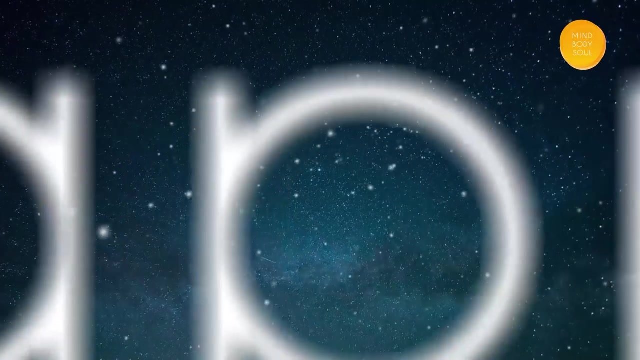 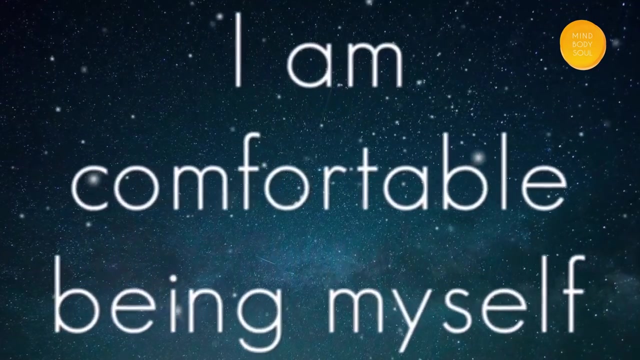 I enjoy good health and fitness. I enjoy good health and fitness. My body is capable of regenerating. My body is capable of regenerating. I love and approve of myself. I love and approve of myself. I love and approve of myself. I am comfortable being myself. 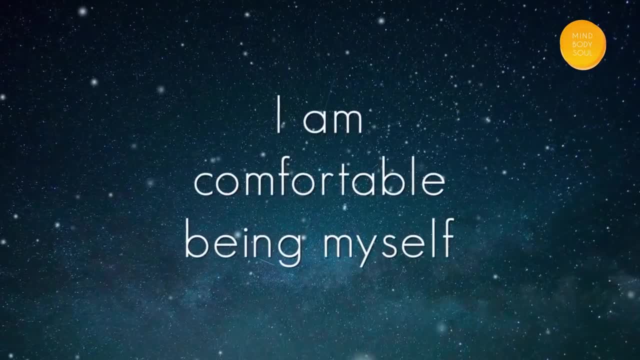 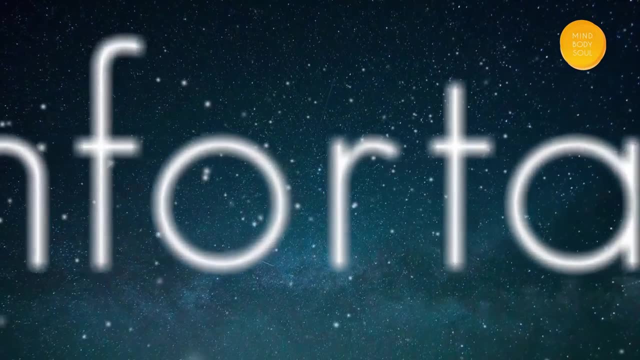 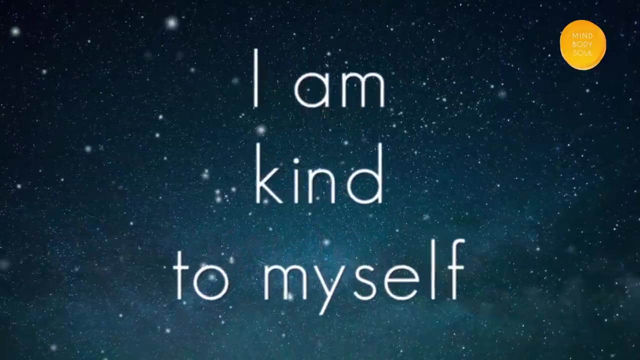 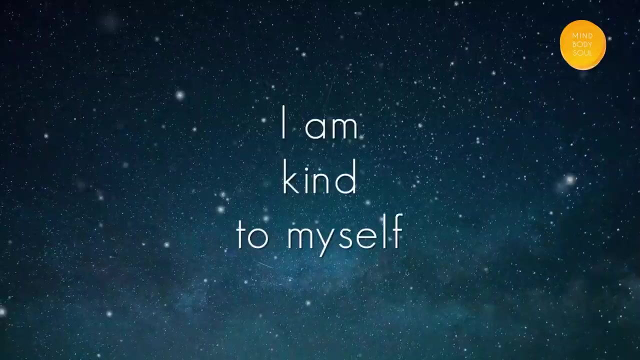 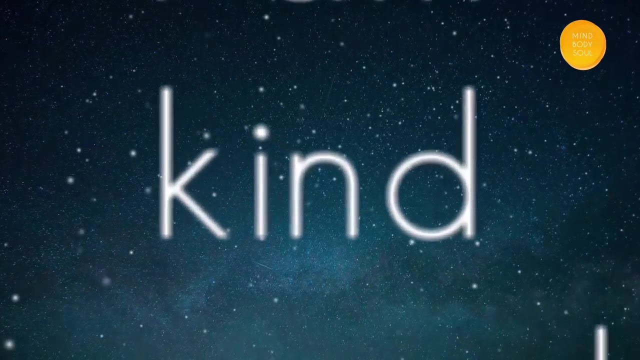 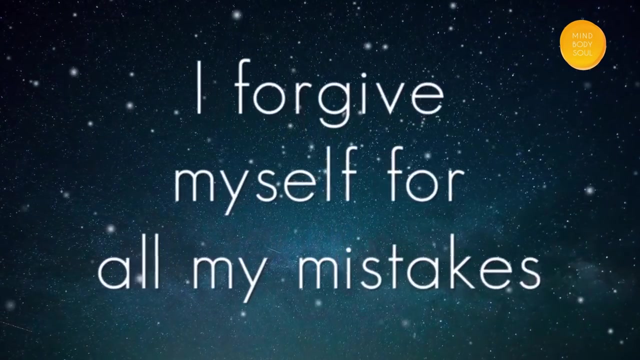 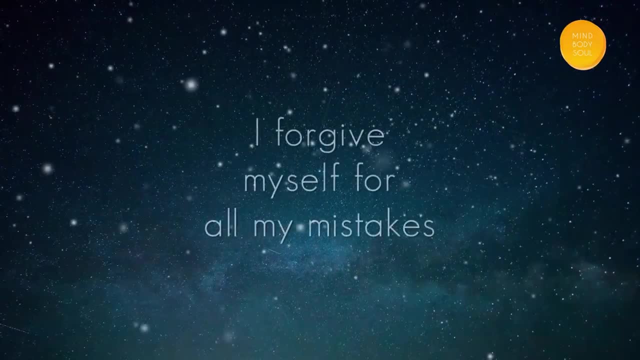 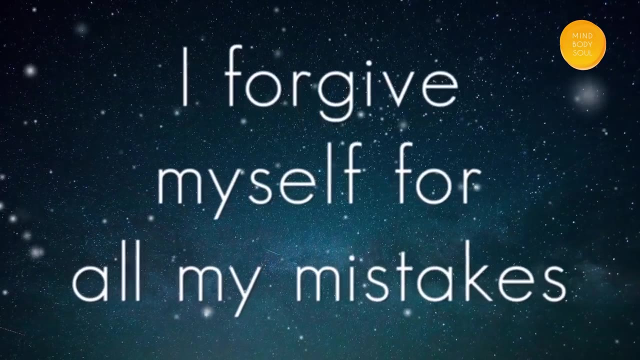 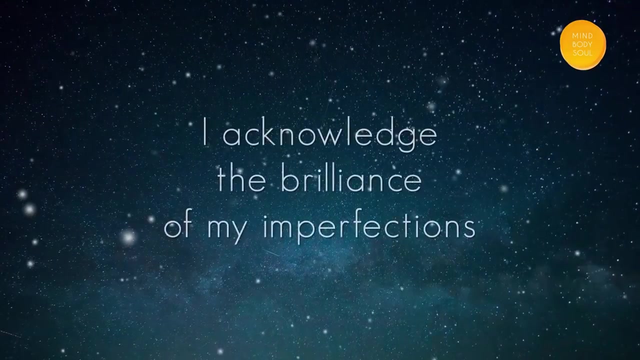 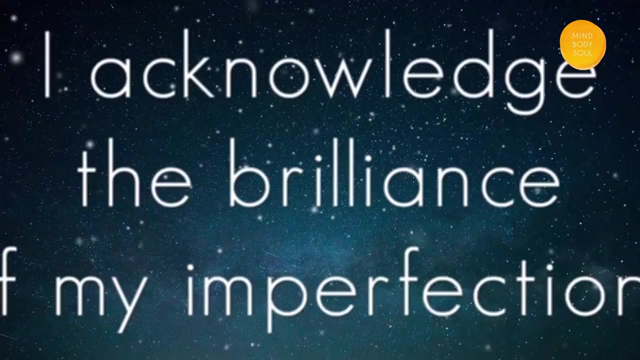 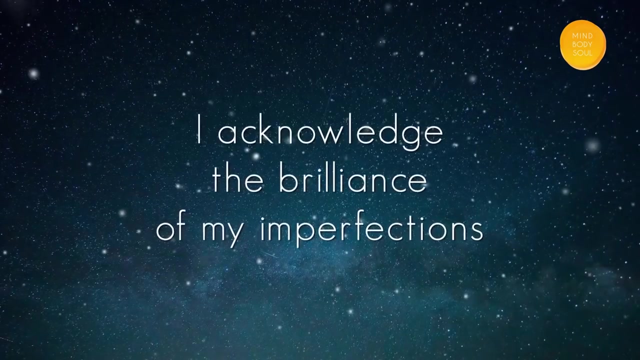 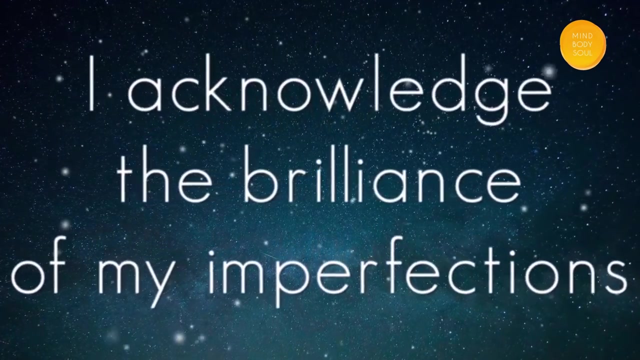 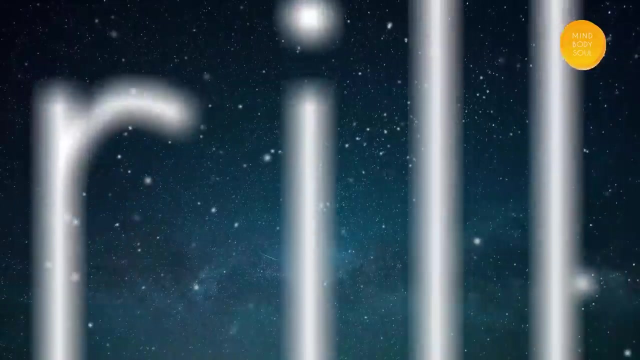 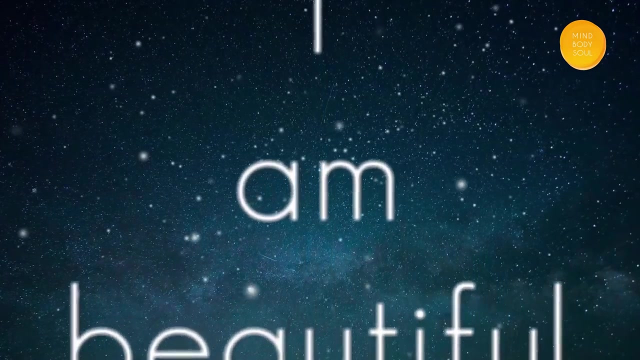 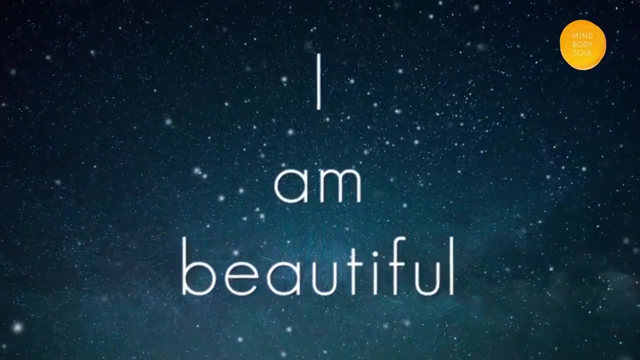 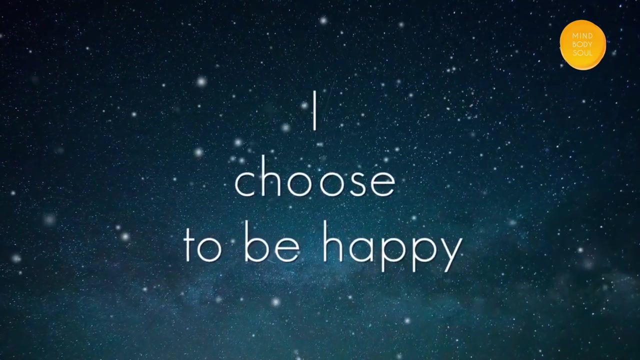 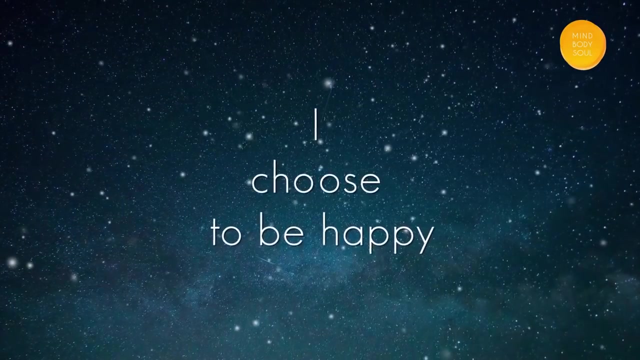 I forgive myself for all my mistakes. I forgive myself for all my mistakes. I forgive myself for all my mistakes. I acknowledge the brilliance of my imperfections. I acknowledge the brilliance of my imperfections. I am beautiful. I am beautiful. I choose to be happy. I choose to be happy. 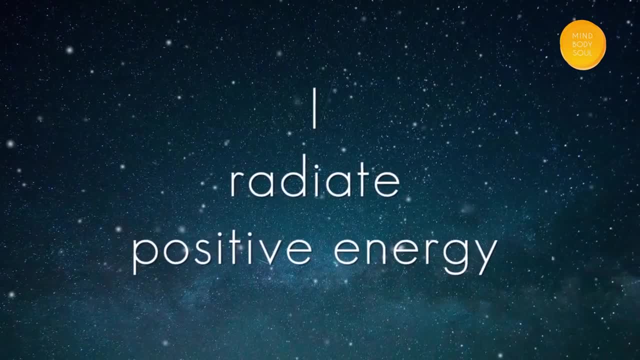 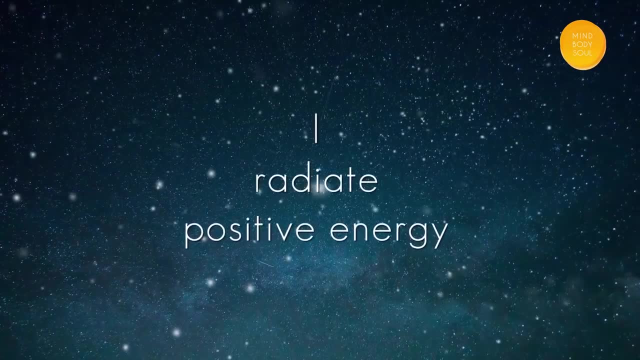 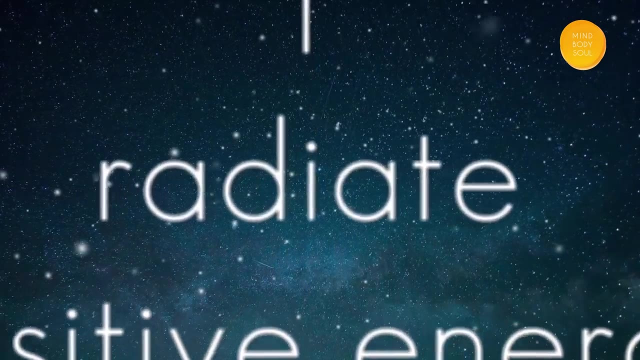 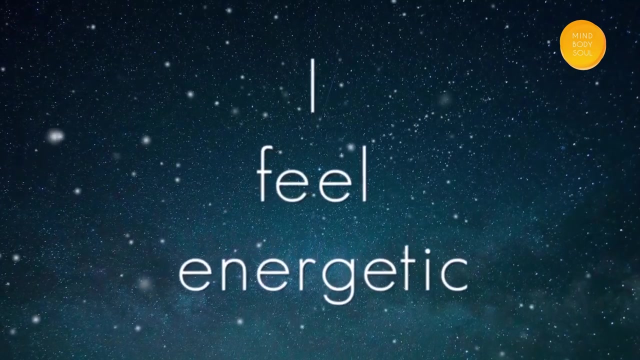 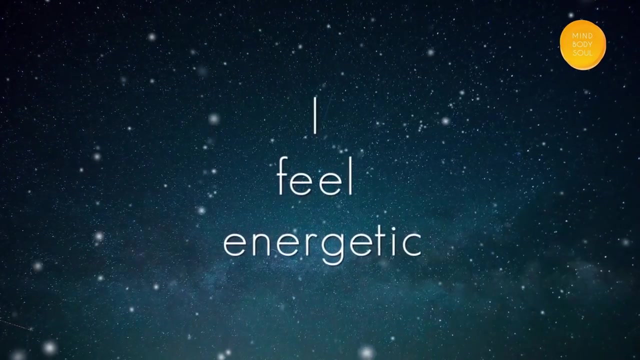 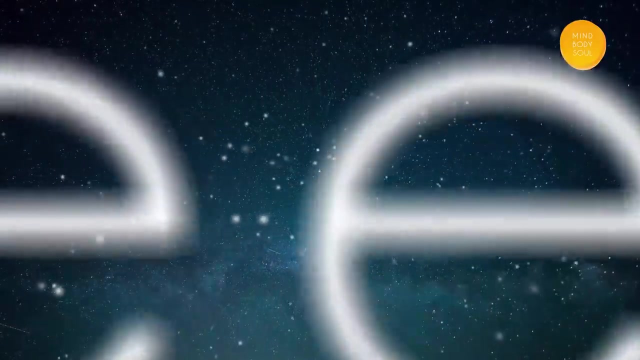 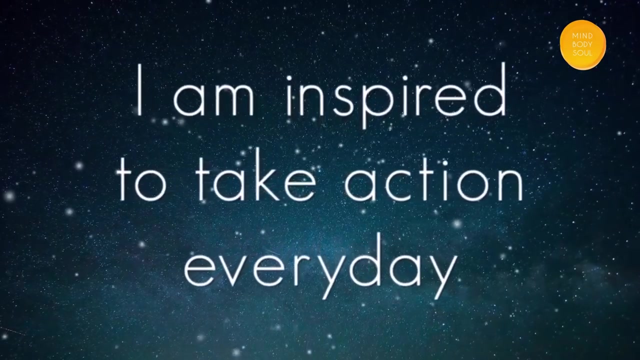 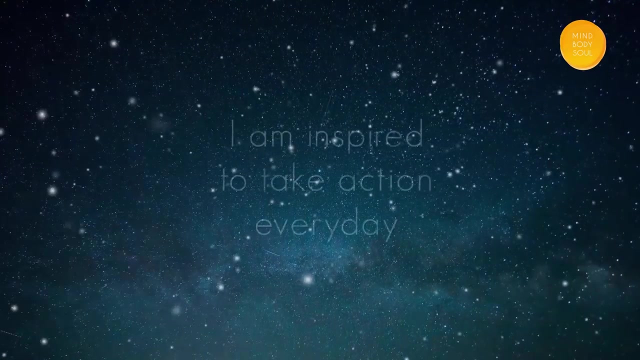 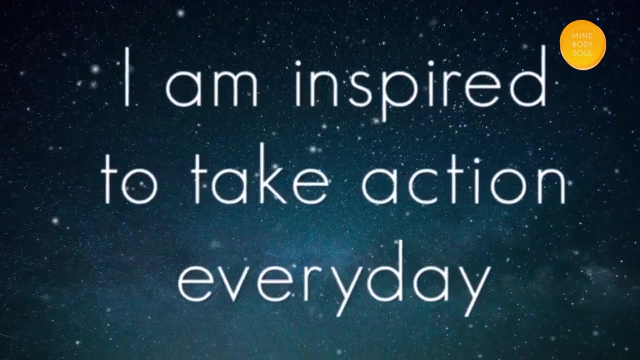 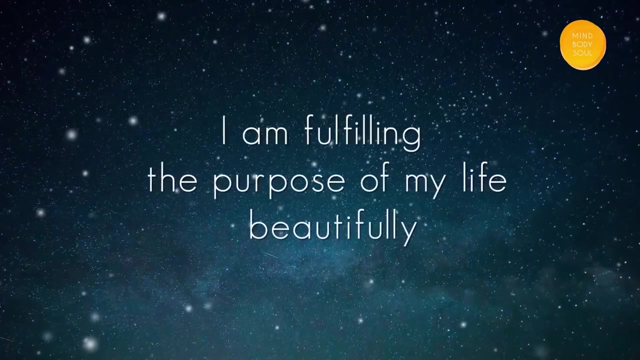 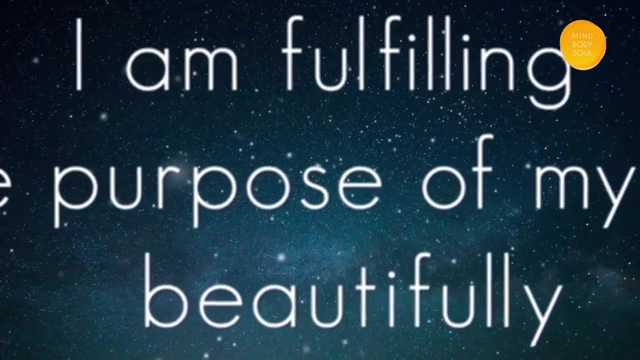 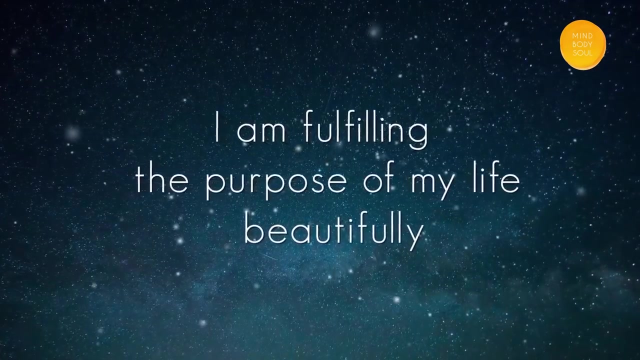 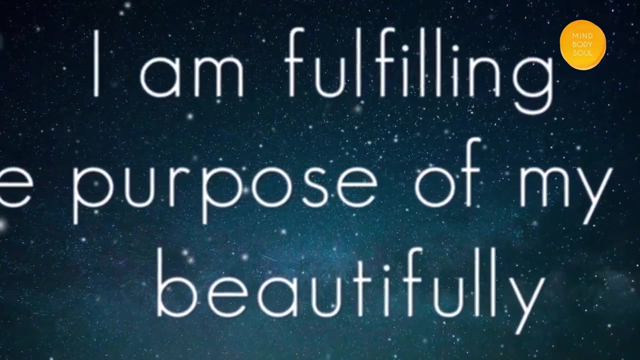